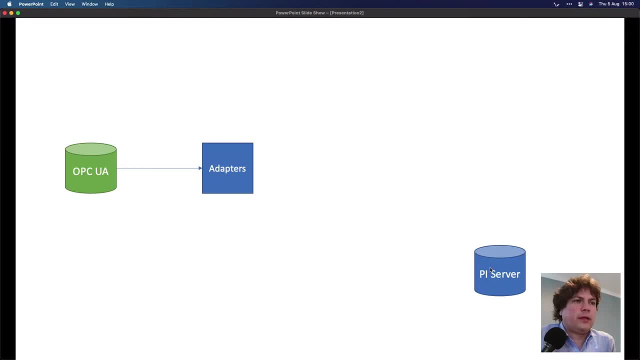 directly to the Pi server, But in this case we have a middle layer in between called the Pi OVBPI. This way, one of the reasons we have this middleware layer is that it allows adapters to be embedded in more complicated network. it doesn't have directly to be access to the Pi server. 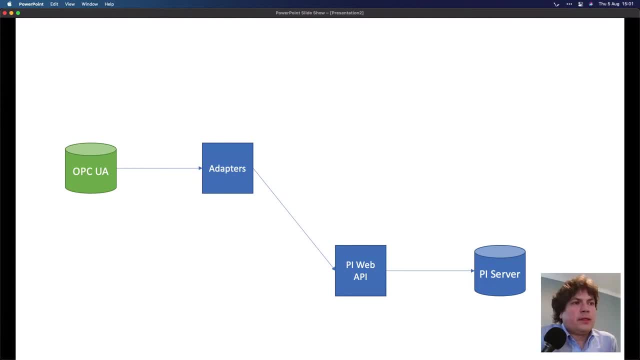 it could be one layer removed from it. The other one is the technology that we use to communicate with adapters to Pi. OVBPI is what we called OMF or size off message format, And it's a technology that we made, and made it for several different reasons. One of them. 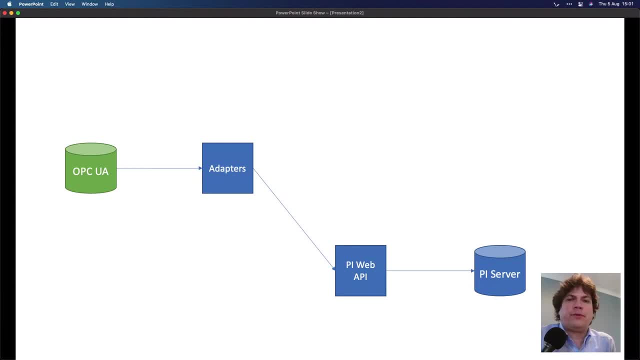 is that it allows us freedom to send the data to multiple different endpoint, not just the Pi server, But we also allows us to send data directly to work clouds, the OSIsoft cloud services, So that's adapters have the ability to send data to both. And when I talk about the configuration, 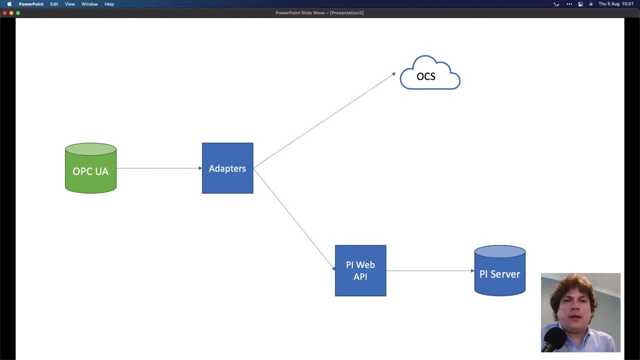 today. I'll show a few ways of doing it, But the primary way of doing it is I'll be using an API that's built on top of adapters And I'll use a tool that's very common for configuring this as a third party tool called Postman. So let me just jump on into my environment. 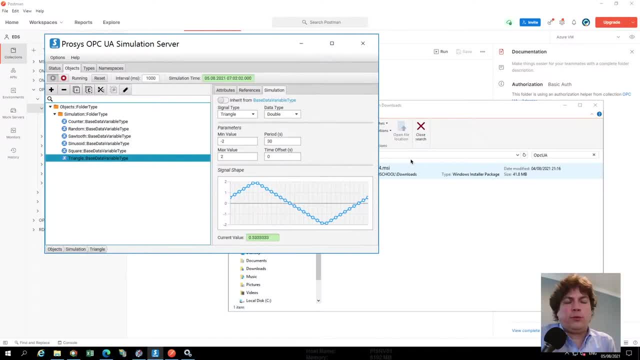 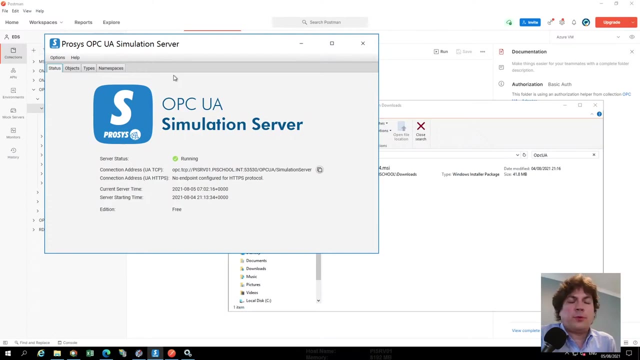 And then I'll start describing how we'll configure it And we'll install the: what we need, what we need to collect the data from, and how to install and configure an adapter. So the first one here that I have. I have a OPC UA simulation service server running on my Windows Server. 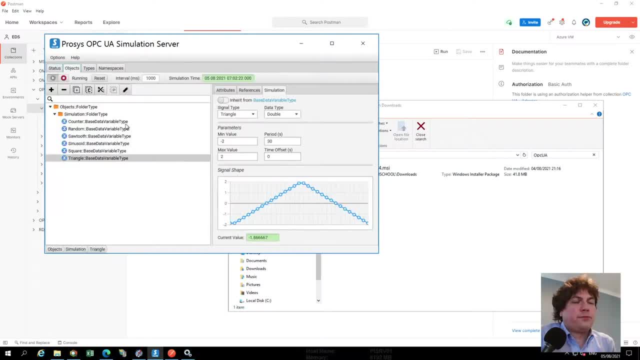 So it's provided by a company called process And it's configured already with a few data tags on the server to do data collections. So I can see there's a few tags, things like a counter, a sawtooth, a random strand, you know sinusoid. 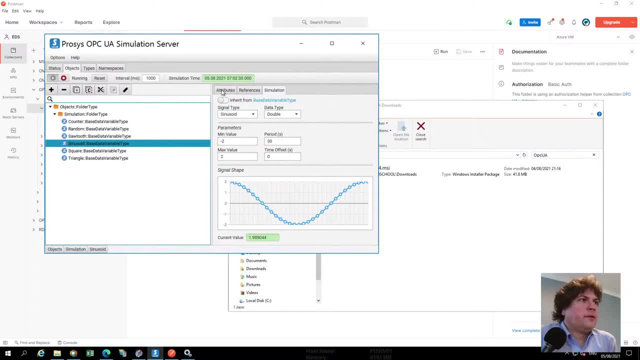 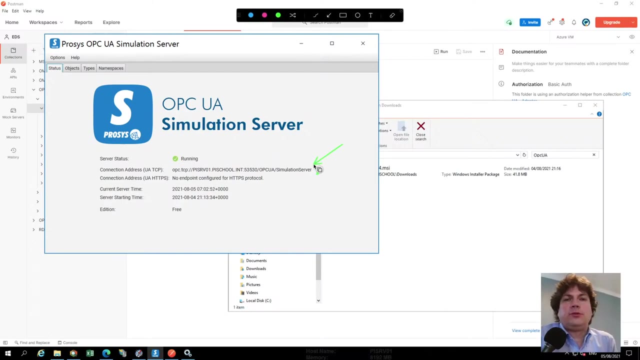 So typical type of values that are being generated. The other important things that I can see is information about you, know their address within the OPC server, UA server, and also, for example, where the OPC server is located. So these two pieces of information. where's the server? 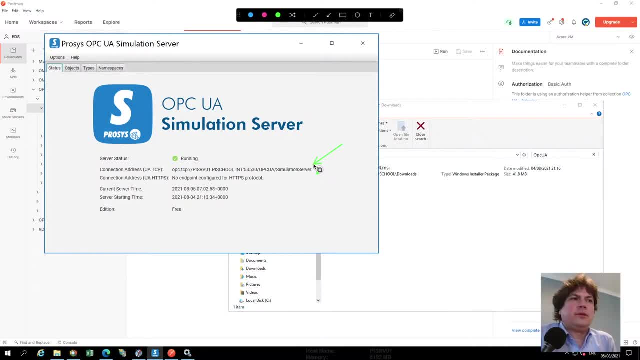 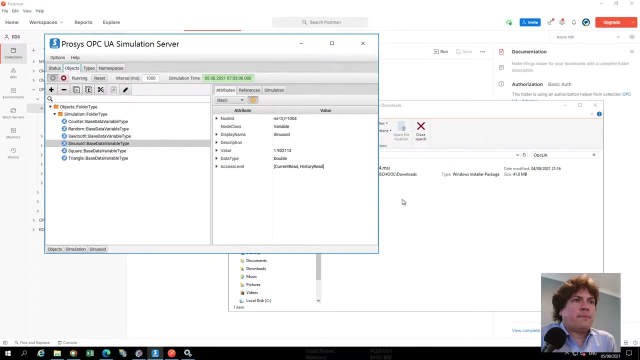 where's the data that I wanna collect? are all that I'm gonna be able to need to be able to configure the data and send it to a PI server or to OCS? Okay, so let me just run first the installer. I just have a simple MSI. 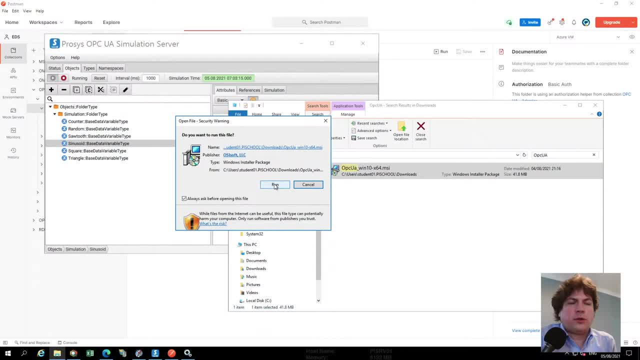 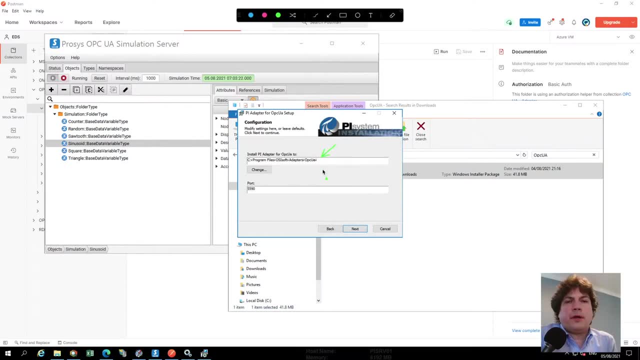 It doesn't have any dependencies. It's simply run on NET Core. It's a very simple installer. The only thing you really need to understand is, like you know where am I gonna install it and which port am I gonna be using. 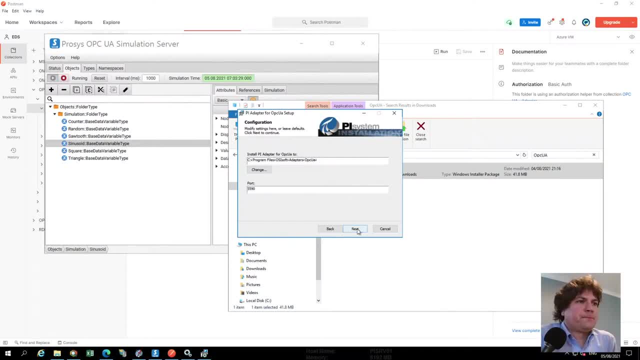 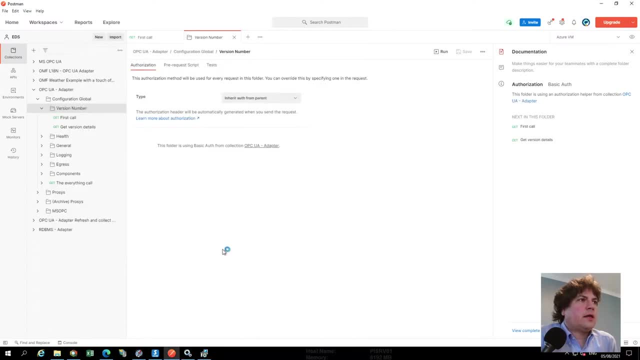 And the port information. we'll see why in a minute And I'll just hit click next, click install, and we'll run the installer In as we're letting this run. I just wanna talk about a little bit about the tool. 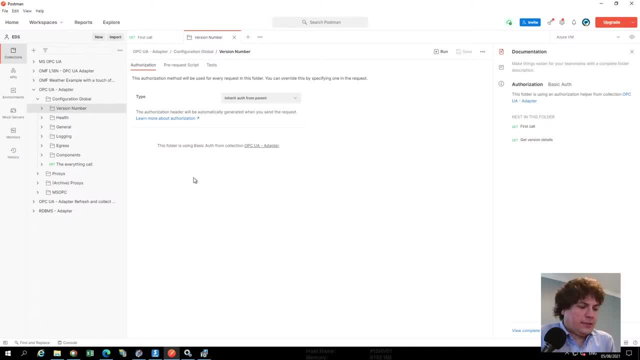 that we'll be using to configure the adapter, And it's called Postman. Let me just set the zoom level up a little bit. See if I can't increase this. It's a little bit easier to see. There we go, Zoom in. 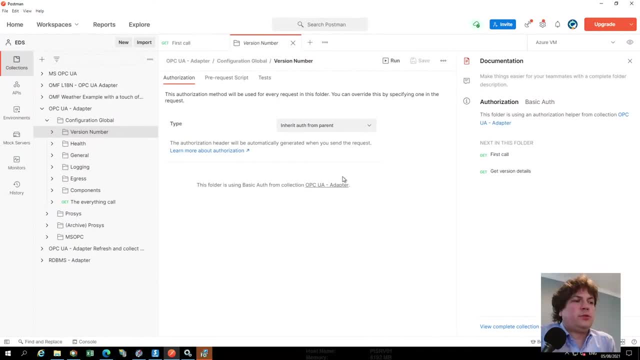 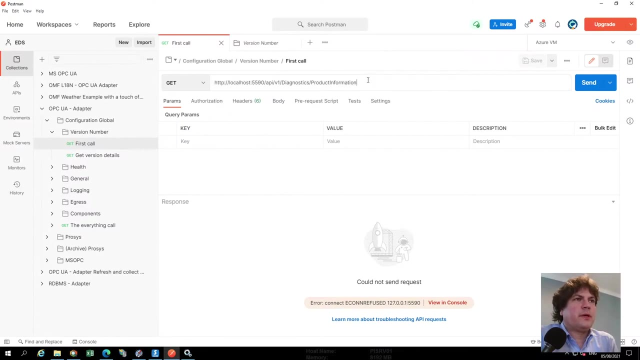 Let me zoom in again, All right. So this is the tool that's very common for interacting with REST APIs, And the adapter is exposed to REST API for configuration. Yeah, it's already finished, And so what does that mean? What does it mean to have a REST API to do this configuration? 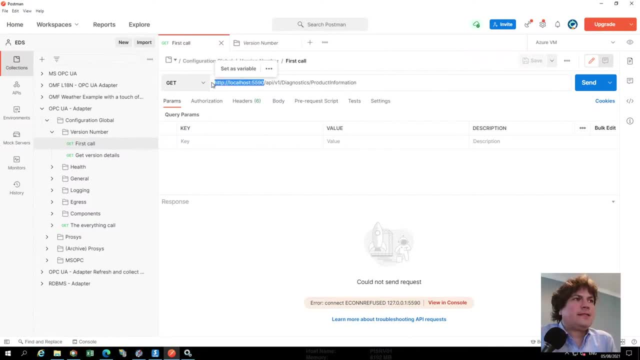 It just means that if I talk to a device- in this case I'm talking to- The machine is locally, So I'm talking to this address and here's the port that was defined during configuration. It means that I can talk to the adapter. 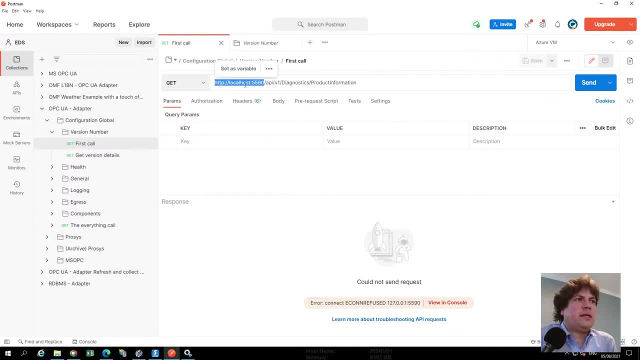 by sending requests to this URL. So my HTTP localhost 5590,. it will answer the information. There's a little bit more boiler to this API and saying I'm using the version one of the API. We do hope in the future we'll add more functionalities. 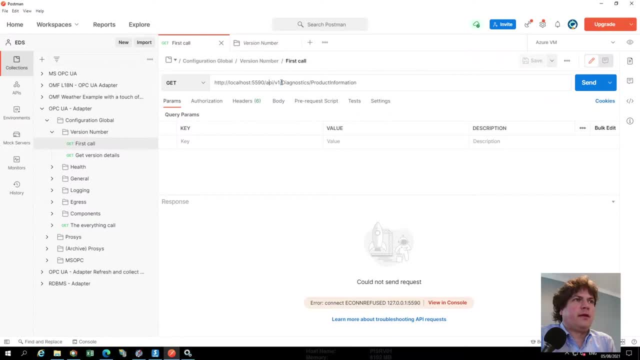 and, but we still wanna retain backward compatibility, which means anything sent to the version one API should still work, even in future releases of the adapters. And I just wanna make the first very simple call which I'll do is I'm gonna get information about the product. 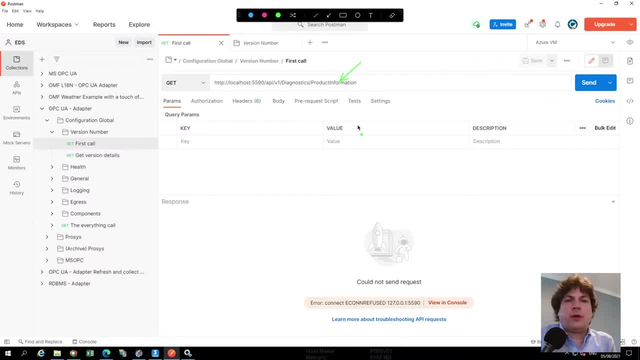 So what is it? The version information with the environment that it's running on and retrieve that from the adapter. To do that as a request, I'll just use the get verb, which means typically means get, retrieve information. So get information from the product. 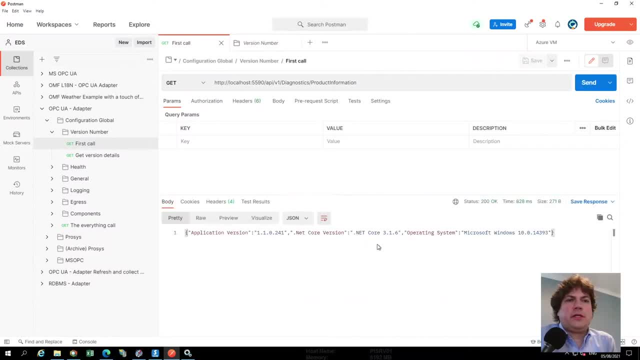 So to do this- I'll just look at it- hit the send button. If the installation went smoothly as it did, I'm able to get information about the OPC UA adapter that's installed on my local machine, So here I can see the version number. It's as I said, it only depends on NET Core. So I figured it looks up the version of the NET Core to be able to use it And also looks at the version of Windows that I'm running, Since one of the design choice of going to NET Core for adapters. 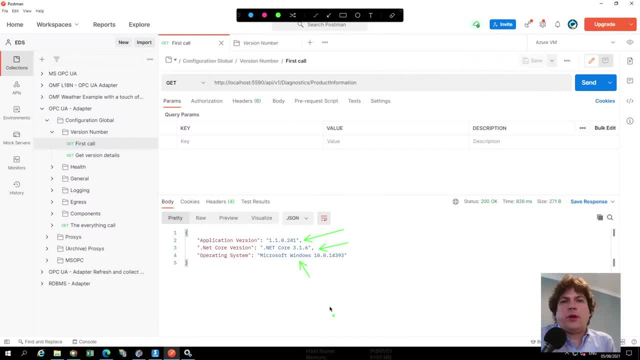 since one of the design choice of going to NET Core for adapters, Since one of the design choice of going to NET Core for adapters means that they run anywhere that the NET Core framework work, And so you'll be able to run them in Linux. 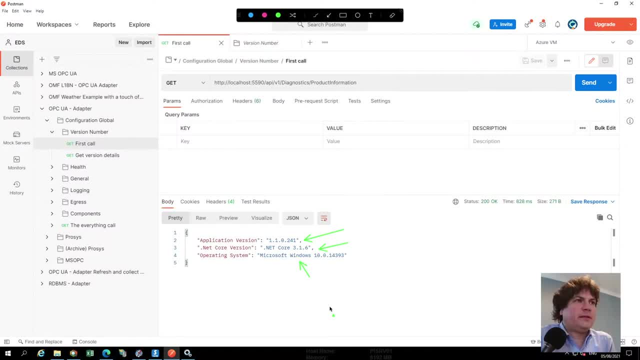 You'll be able to run them in containers, So you have a lot of flexibility inside of them. Okay, And here I want to start configuring them. The first thing I'll notice is that the kind of this URL that I'm using- http//localhost5590.dpiv1. 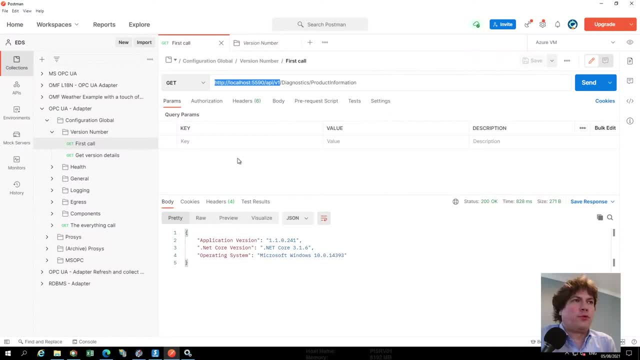 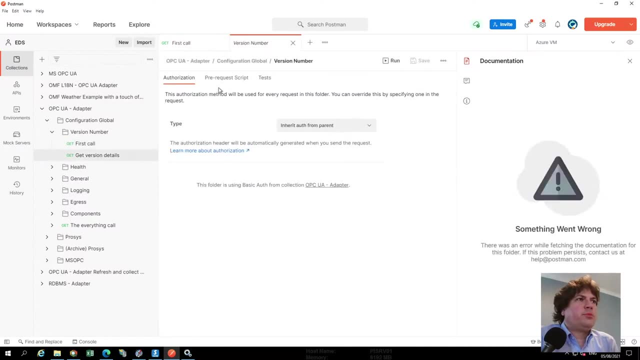 is the kind of the root URL that I'll keep using over and over again, And so what I'll do is just to look, simplify the URL, then I'll be interacting with it. just put this URL information inside of a variable here. 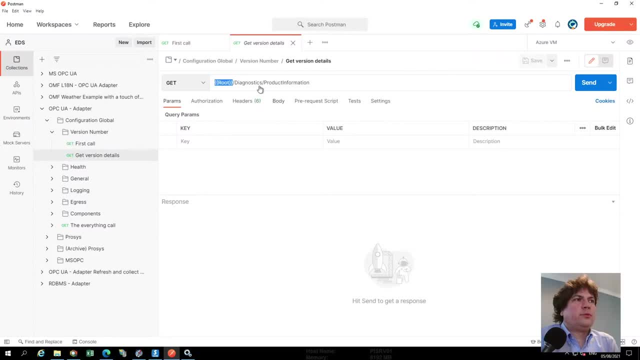 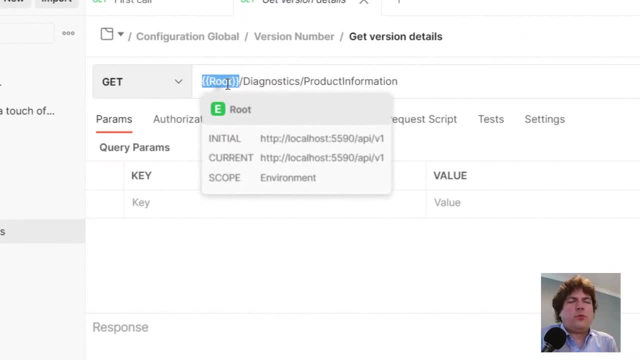 So I just have a variable called root and the root variable, if I look into it- let's just zoom in- it stores this variable here. So I'm always thinking underneath there's a full URL that I have to call it, but there's a part of the URL that's always fixed. 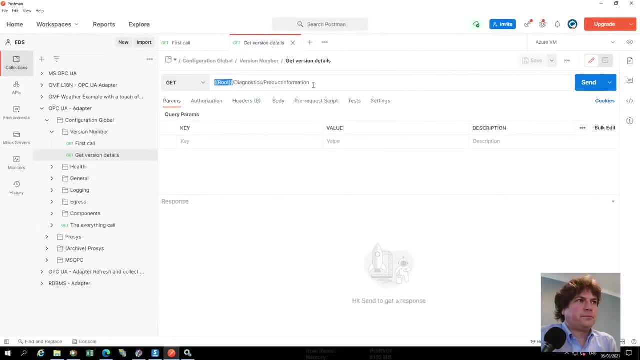 So I'll just use only verify this fixed information so I can get send. so I can get send And it still retrieves me the same information about information. that's done Now the question is: okay, how do I get this part of the URL? 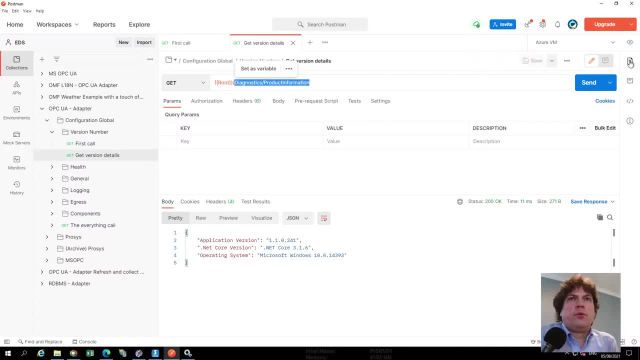 So the part that's not fixed, that's dynamic. How do I look at it? What I do is there is documentation that we can get, So here's just a documentation that I've attached to as part of Postman, But if I click on, it will give us to the documentation. 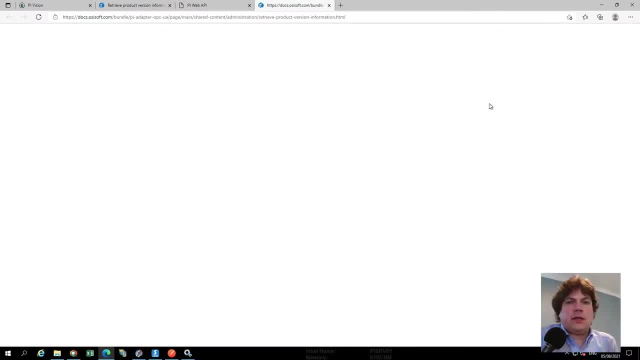 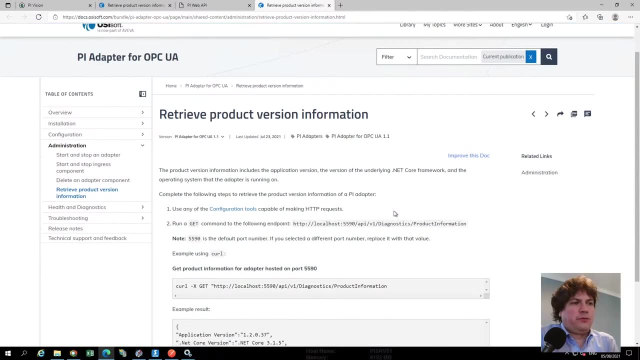 that's part of our website And if you look at this documentation there, you will see all the calls that we can make, The outputs that are expected. what are the expected inputs? all the variables are gonna be defined here. So this is again: how do you get information about? 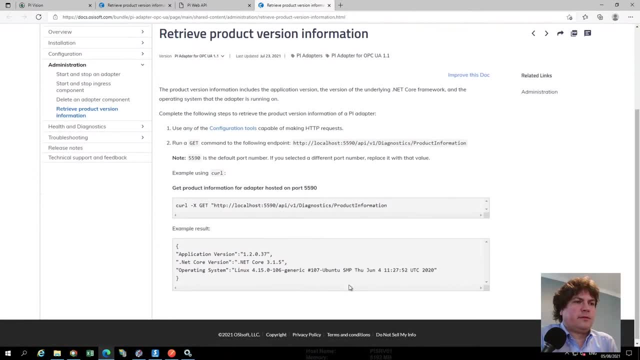 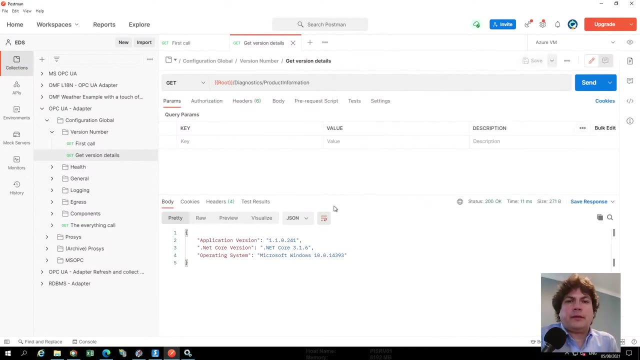 you know product version information, So what should I expect? And there's a nice sample. So if I was running it on Linux, this is the result that would have gotten. Okay, so let me go back here, Let me go back to Postman and I'll start configuring it. 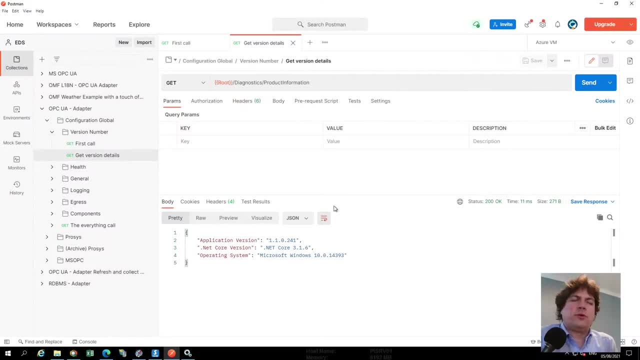 I'll go from, you know, the very, the broad definition, So configurations that are available to every single adapter, and then go to the ones that are specific to the OPC UA adapter. So the first thing is I wanna talk about health information. is we can get the information about the adapter? 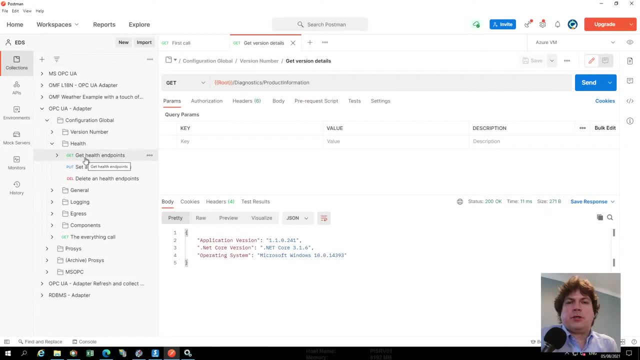 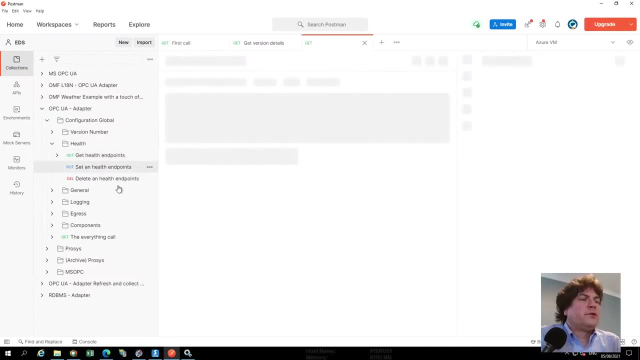 Is it running correctly? Is it running into issues? How much you know? this space is left. All these type of information can be pulled from the adapter and sent to the PI Server. So the first thing here I'm gonna do, a request- is I'm gonna say: 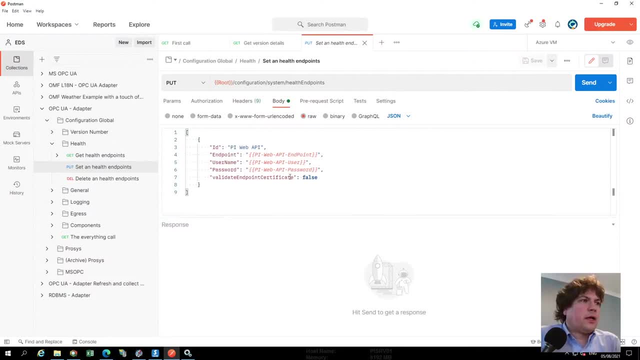 I want you to send this health information. I want you to send the information to this PI Server here And I just I have the information here- just says: what do I wanna call this health endpoint There's gonna be, maybe you know. 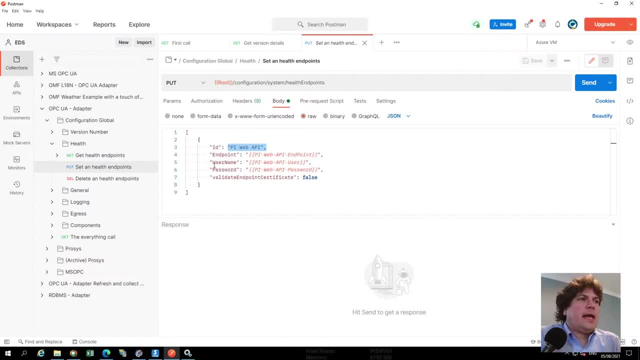 you're gonna send it to the name of a particular PI Server. You can use that name And it needs to authenticate to this instance of PI Web API. So I have to send the health information And so I have to tell it where is this PI Web API endpoint. 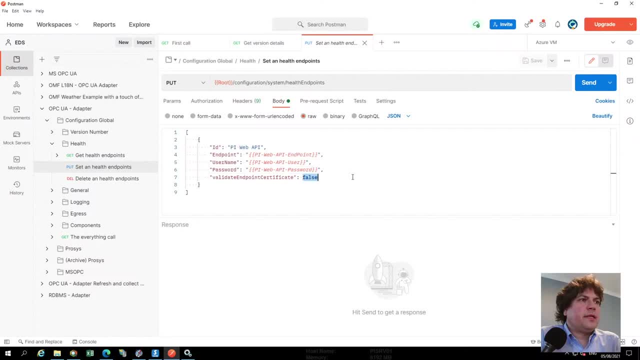 username and password to be able to authenticate. This last one is the validated endpoint certificate. is information about. do I wanna trust a certificate that's part of PI Web API? So any communication with PI Web API is over HTTPS. So there's a question: is this gonna be a good or valid certificate? 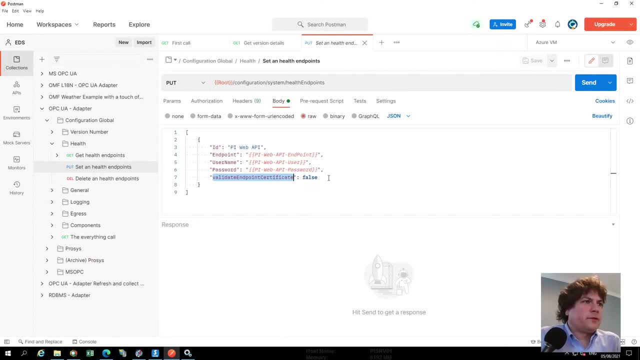 or not, So we get the option of not doing it. So, actually just for demonstration, I'll just actually not specify this field and let's see what happens. So here I'm just gonna send the endpoint, set the endpoint to this field here. 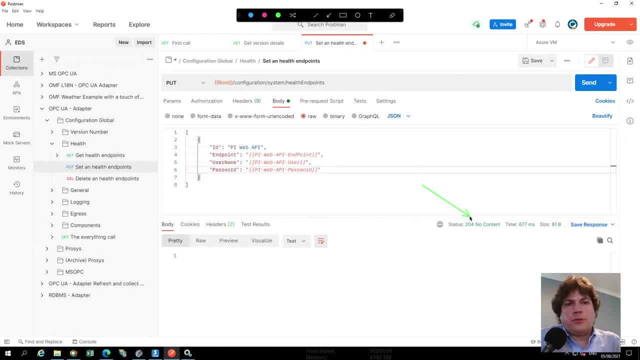 Now what PI Web, the adapter, returns to me is this code of 204.no content. It simply says there is no syntax error with your message. I've accepted it And now I'm working on this request And I can look at it. 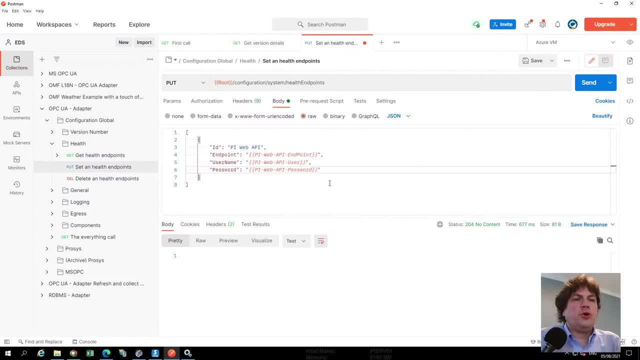 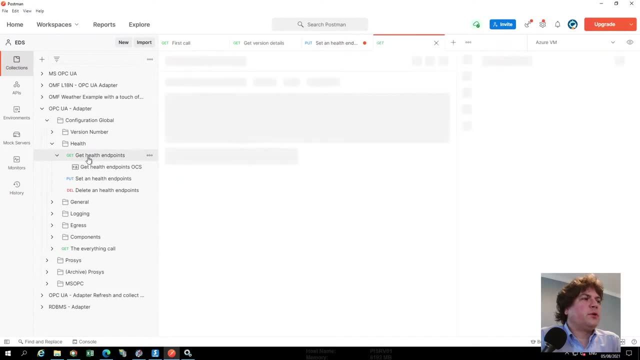 I can look at the adapter configurations to know if it was accepted or not, So to see how it was stored or not, by just retrieving, querying the information of the adapter here. So I'm just gonna go instead of getting putting a put. 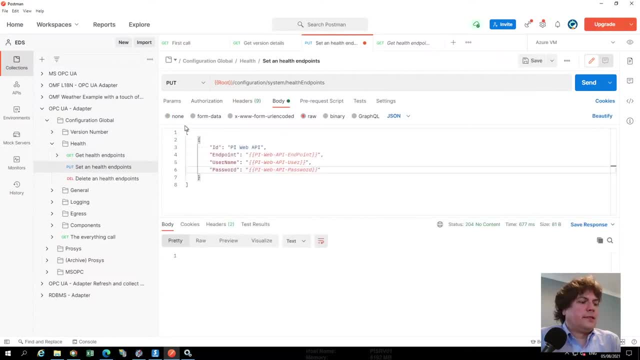 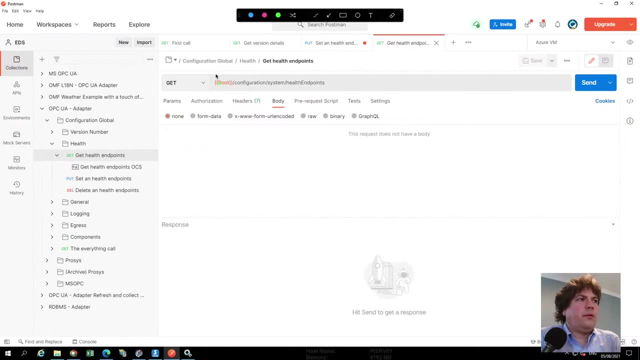 by sending the information. sorry, go back. So here. I sent a put So, which means I'm sending the information to the adapter. I can do again here the same URL, but specify get. So I'm retrieving what is stored. 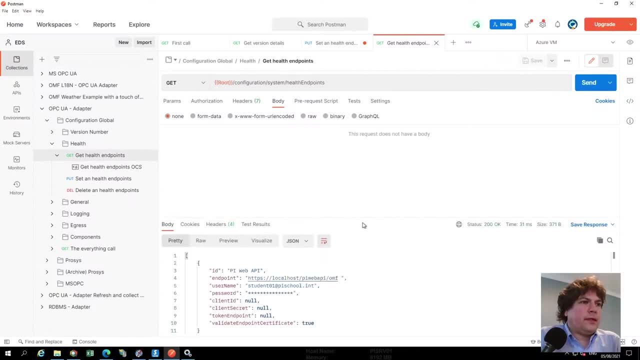 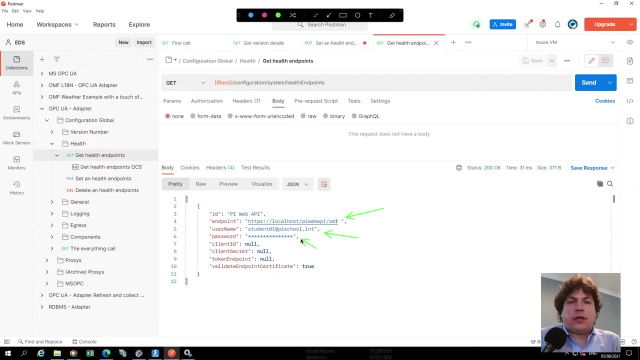 I'm going to put the password within the adapter, So I'll do a get And I can see the information that I've sent. So these were the pieces that I had as variables within Postman. So where am I sending the data, username and the password? 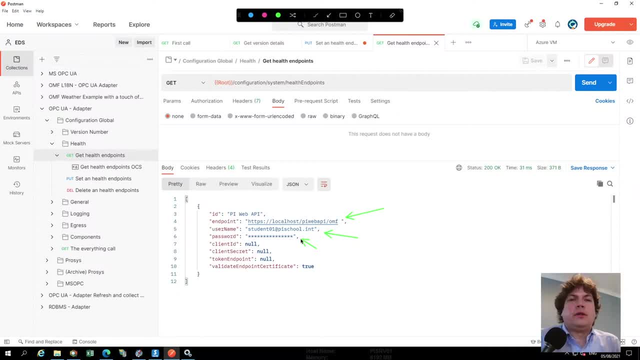 The password is replaced by star because it's encoded locally. So the information, the original username and password, the original Windows password, is just gone. It's just encoded in a way that I could. the adapter is still able to use it, But anybody who's looking at the system? 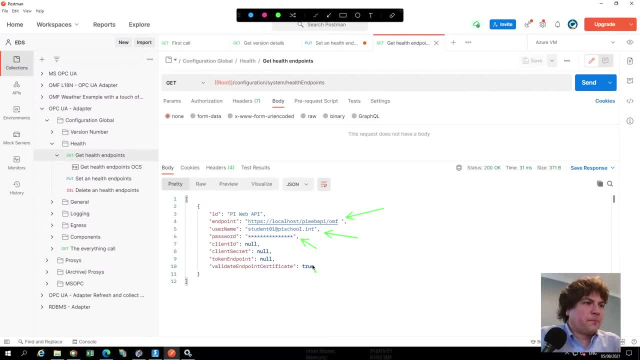 is not able to figure out the name, So they're not stored in plain text somewhere, And I can see that it has this value that was previously defined. the validated endpoint certificate was set to a default value of true, And then I can see these other things here. 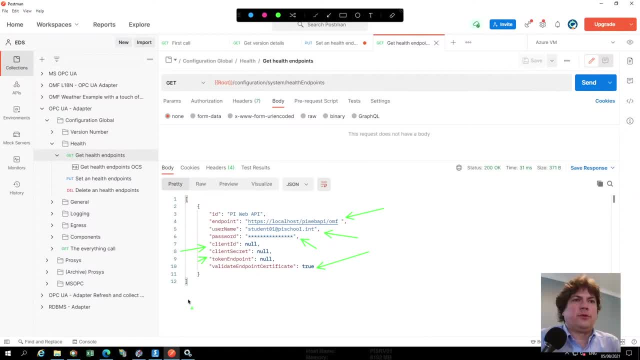 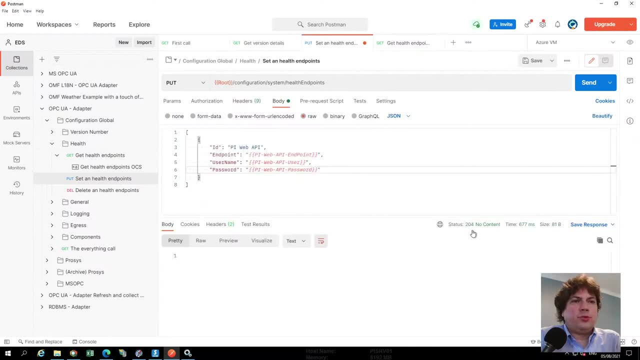 which are related to OCS and are set to null, because I'm not sending data to OCS, I'm only sending it to the PI Wave AVI here. So I wanna try to understand this 204 a little bit better. So what I'm gonna do is go to the logs. 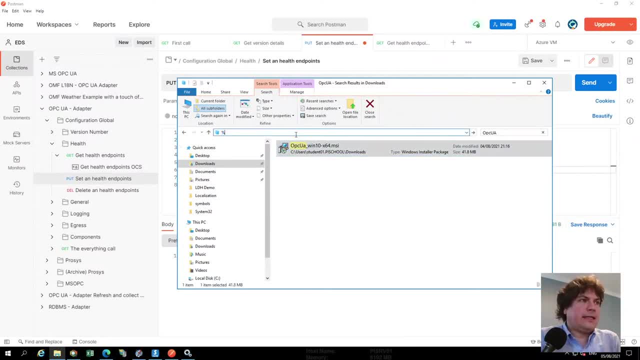 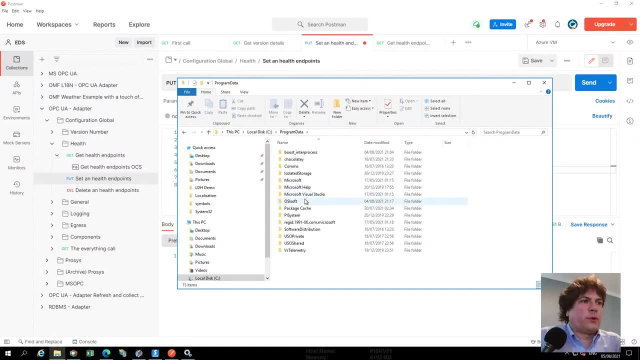 and the logs are gonna actually tell me how is the adapter actually processing this data. Is it running into any issues with going over the request that I've sent it to say, send health information to the server? So I'll go to where the logs are. 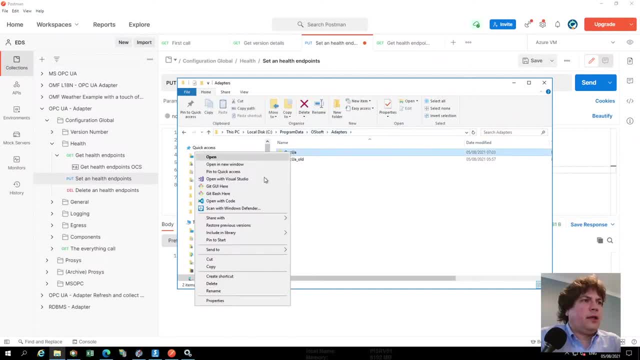 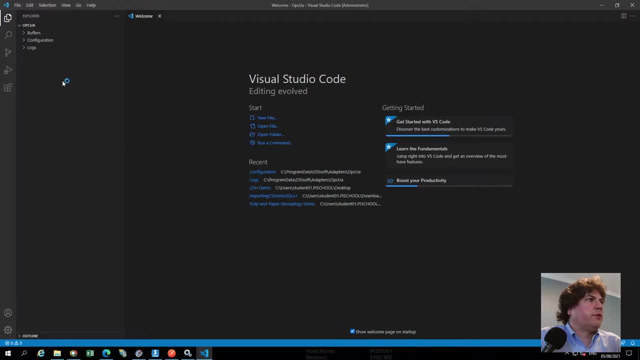 So I go to program data OSIsoft adapters and I'll look at this OPC UA folder And I'll just open the entire folder to look at the what's contained in the configurations that are there. So the first thing is I can do. 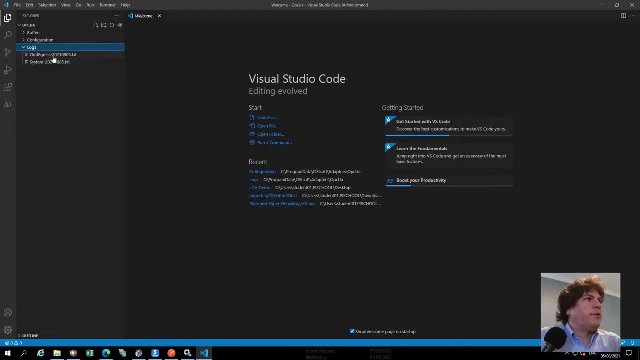 is. I can look at the logs here, So I have no OMF egress log and OMF egress is just like I'm gonna try to send data to somewhere, but so far I'm not sending any data, So there's nothing there to be configured. 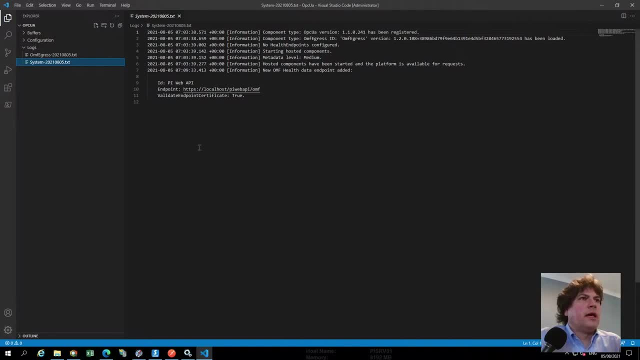 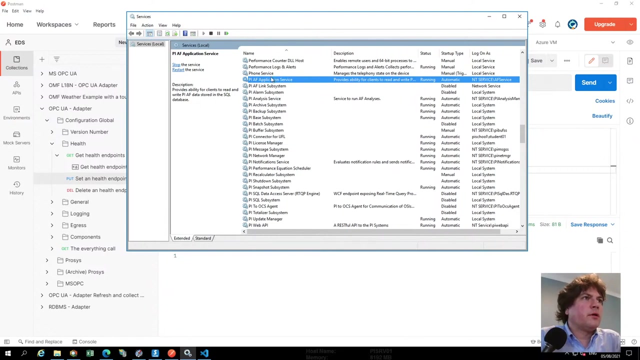 And the system is there and it's configured to do it. Okay, so there, it retrieved an endpoint To retrieve data. Okay, So let me just quickly verify. And so the adapters are running as Windows service and I can see here again that it's currently running. 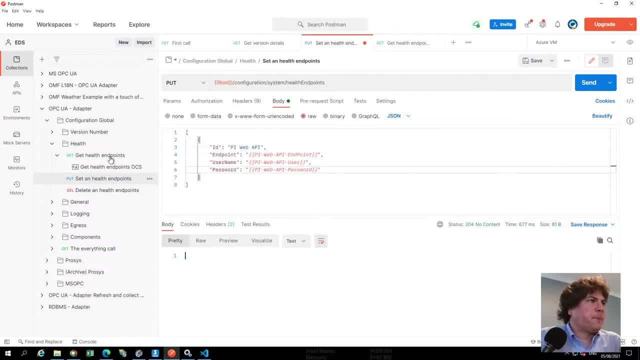 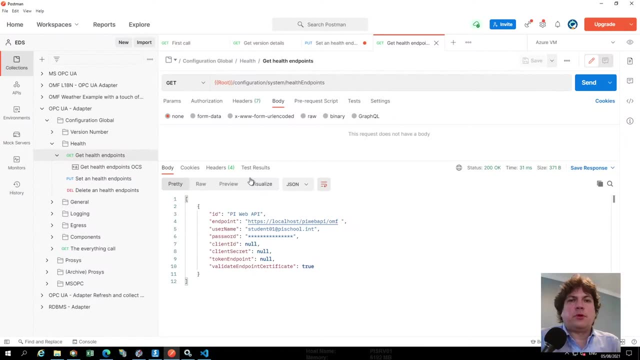 So if there will be health data to be sent, it will send it there. The other thing here that I'm using functionality of Postman that I use very commonly when I configure adapters, just for as demonstration purposes, is I also kind of solve a save the request. 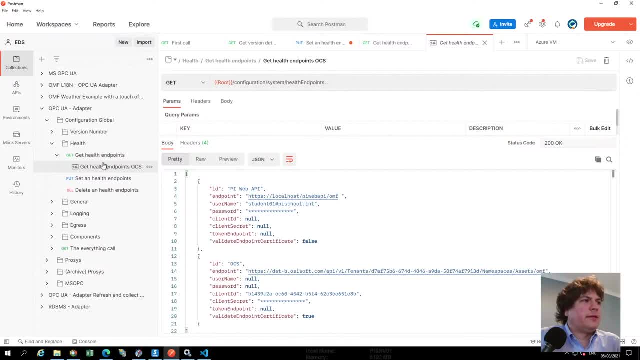 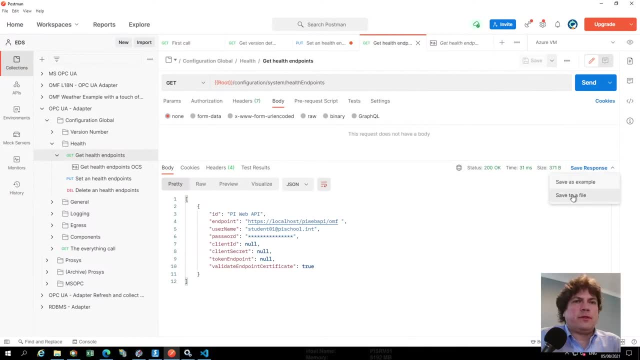 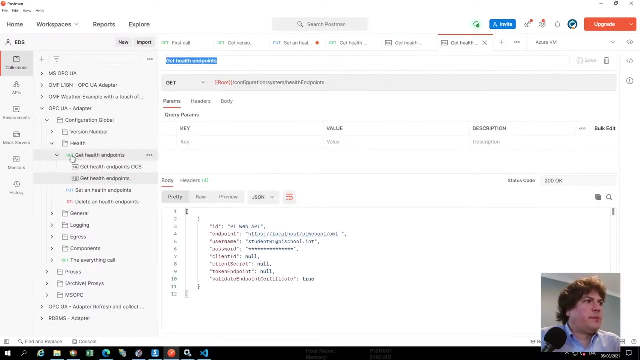 that I have into kind of the like samples here. So, for example, actually I'll do this for this. This is my current configuration. I'll just save this to save as examples. It saves it as a kind of a sub object of this request. 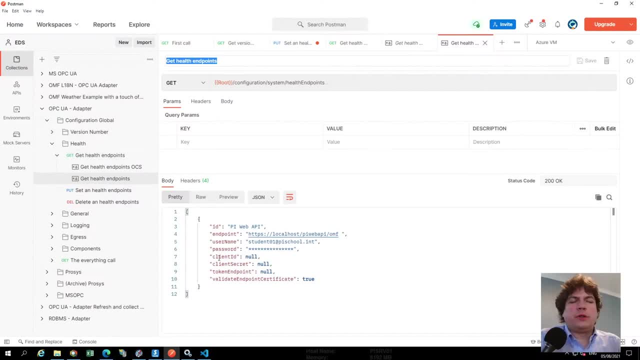 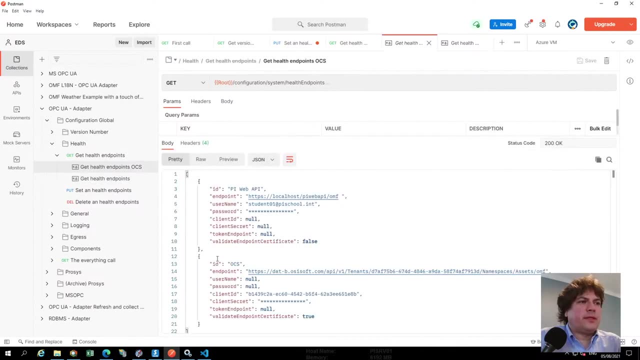 So if I ever wonder what should the result be, I can always look back at these notes here And I put for myself In particular, I was sending health data to OCS at one moment. And if I want to look back at what was the configuration, 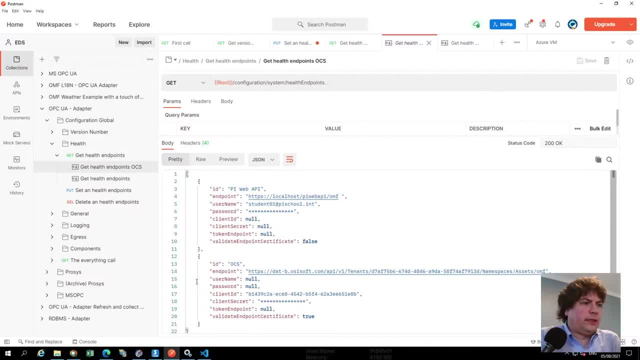 when I was sourcing it to OCS here. I can always just quickly go back and look at one of these saved requests and look at the data. Okay, I was sending it to this OCS tenant And, within OCS tenant, I was actually sending it to this tenant here. 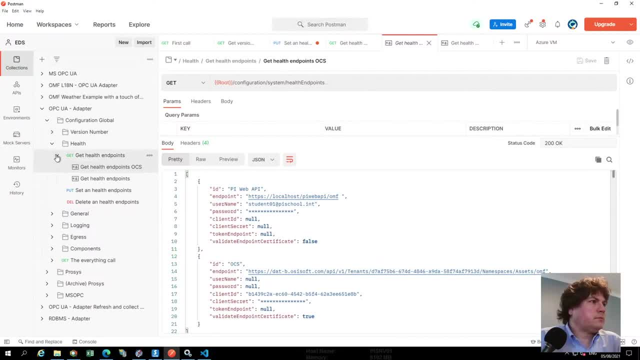 to this namespace here, Okay, so the next thing I wanna look at is: okay, so here. what I'm doing here is I've done a request, a very simple request, to just send data to one endpoint here, And what is kind of curious about it is 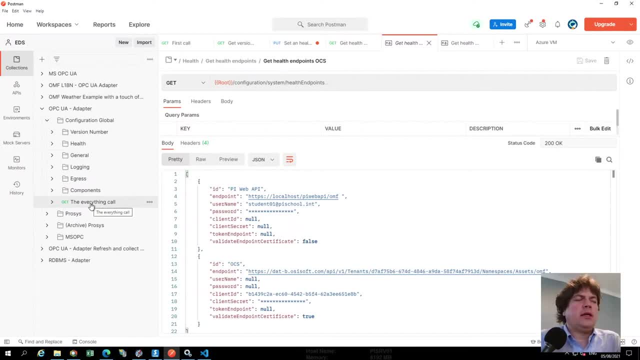 okay, what's kind of interesting is about it is: I've done just kind of an incremental change to the adapter: Where will I send data to, But how people will go and configure adapters in the future. Well, that's just one way of doing it. 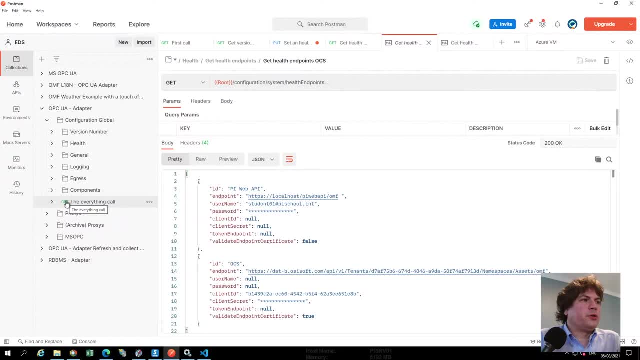 Do we do these incremental change? Is that the way that people are gonna do it? Or they're gonna be, for example, just building a big JSON object that has all the configuration and send it to it, Or will they use some sort of tool? 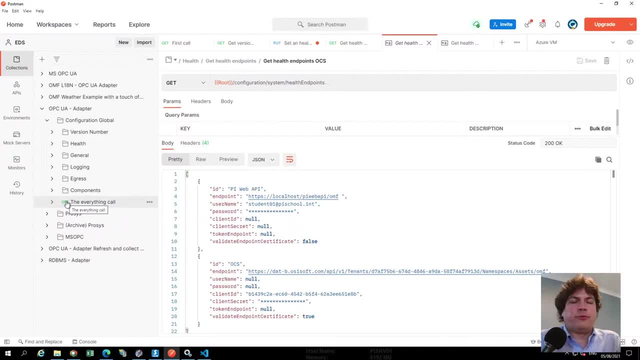 that automatically configures the adapters. So there are lots of ways of provisioning software. Will they use that, Or will they use kind of a command line application that we also provide? I'm not quite sure. So there is a lot of these options here. 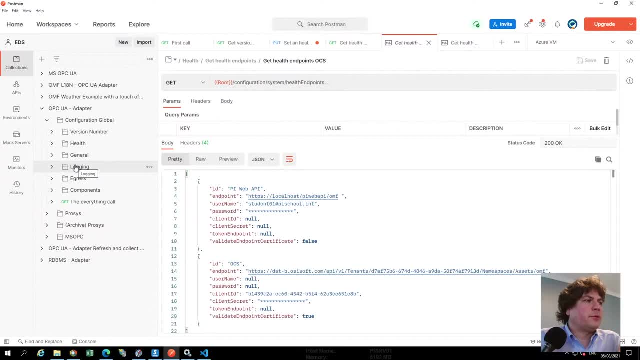 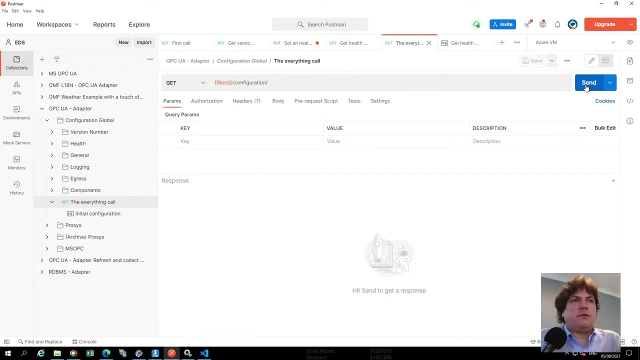 I do prefer this kind of incremental approach to configuring an adapter, but the other options are valid. So, for example, if I wanted to do a gigantic configuration aio, a big JSON object that contains everything that I want to do, I can also just create that object. 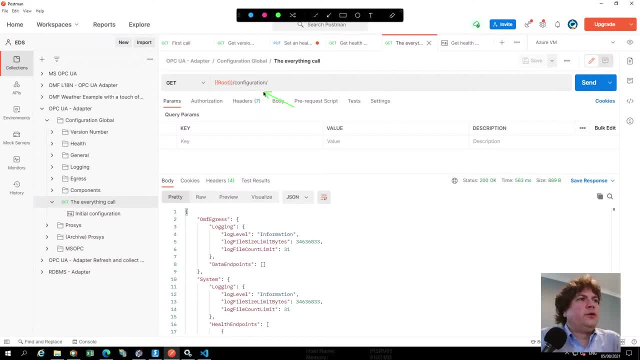 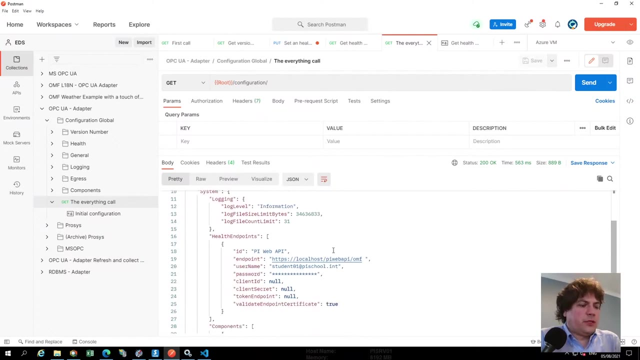 and send it to the adapter. In that case, the URL that I would use is simply the route URL slash configuration. It's very generic. it just says: okay, well, give me everything that you have, and i can see here that it already contains some of the information that i have configured, some of the, for example, this help point data. 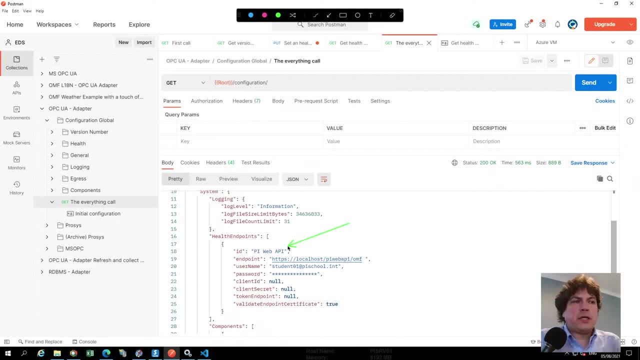 here. it's already there, so as i'm building up my configuration, i couldn't always look at the global configuration, which is an object that contains all the configurations for this adapter, and this single file will contain the record of everything that has to be done to configure this. 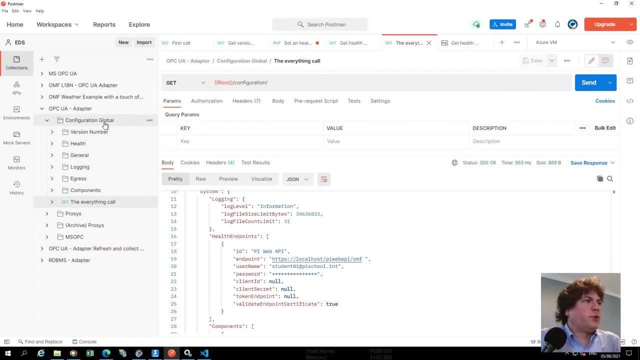 adapter, but i'll just continue on here. so i'm continuing here with these kind of these global configurations- so the configurations are generic to the adapter- before going to a configuration of this particular opcua server that i want to collect data from. okay, so the next one is: i want: 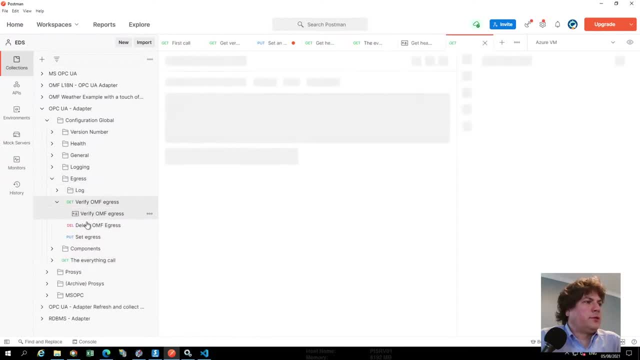 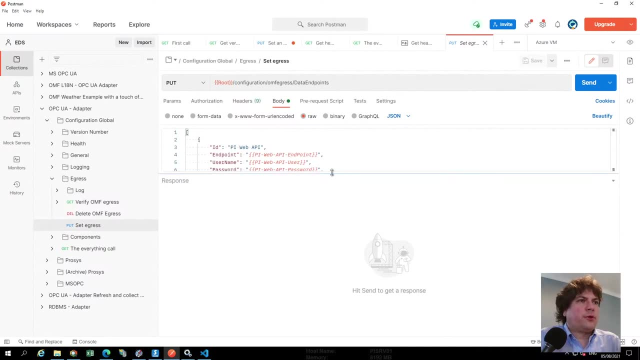 to specify where am i going to send data to. okay, so i'm going to send data. so, again, i have to do. it's going to be a put request and i'm going to say: this is a new configuration that i'm going to be using to send um, you know, to. 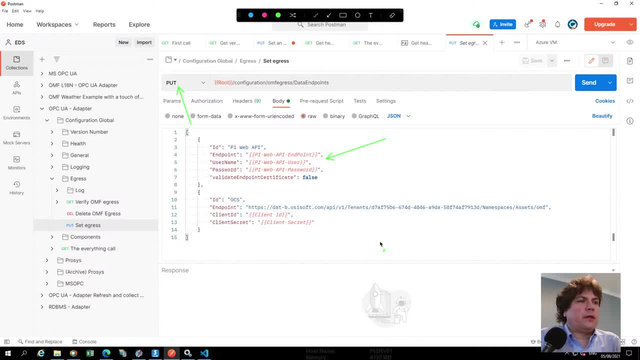 send data and i'm going to have to specify where am i the data i'm going to be sending. in this case, i'm using both piwave, api and ocs as targets to send the information. and the other point is: okay, yeah, into the url. unsurprising again. so i'm sending data by omf. so the the urls contains omf. 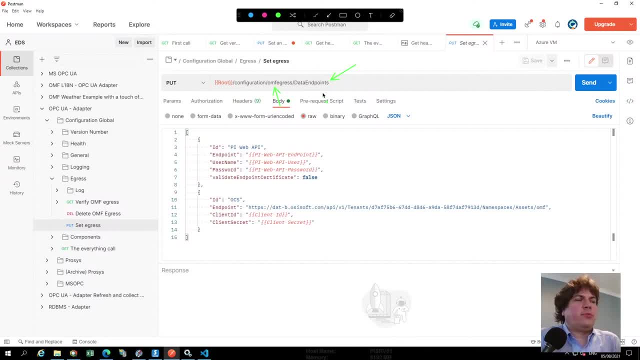 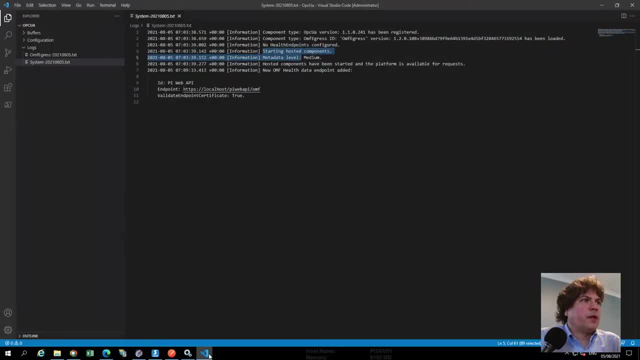 egress and actually my data is going to be sent there. so if i just hit send, it will then start sending data once it actually is configurations here. so here i can see that i have in my logs, i can see that i'm sending data to these two environments here. 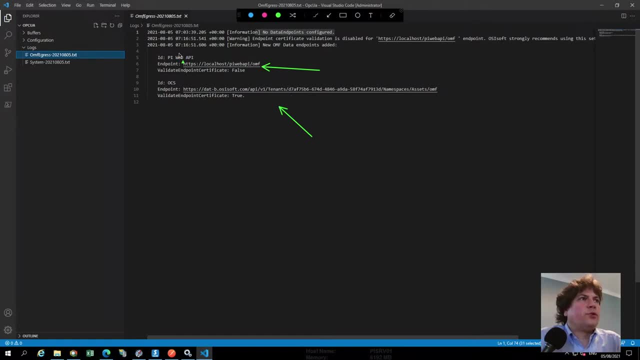 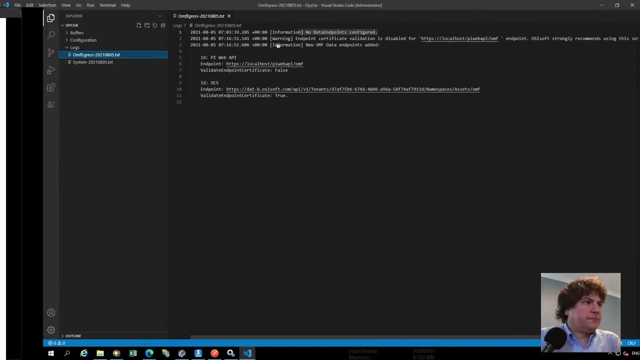 and there's also a new warning settings here that tells me that i've disabled security on this endpoint and but you know, osi soft doesn't support that. so that's kind of a good thing. so that's kind of a good thing of a typical warning, but i'm kind of at the moment i'm ignoring the warning here. oops, okay, actually. 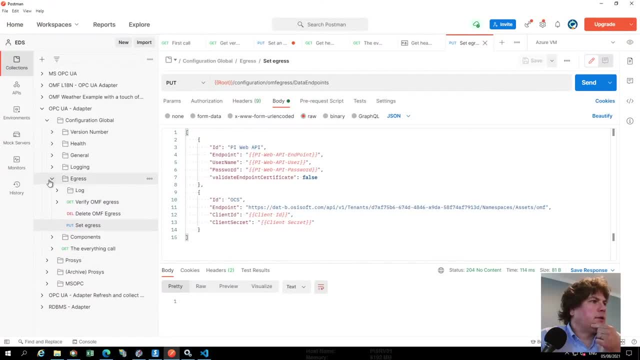 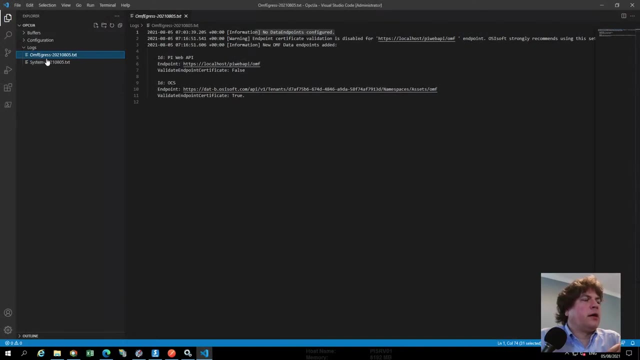 yeah, all right, and so this is good. okay, actually, let me look at the another configurations. here is i. there is many types of logs i can set up inside of ocs, inside of the adapters. so here i'm looking at, uh, the the two logs that were created locally. so there's one for 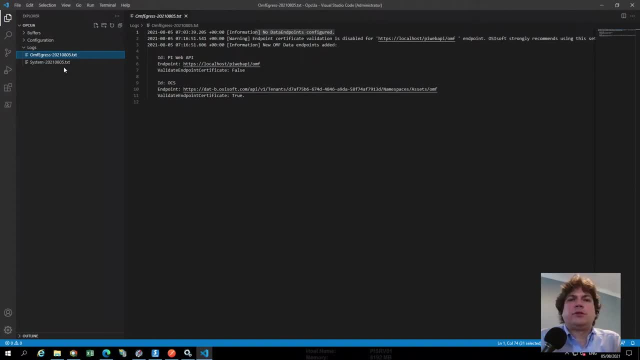 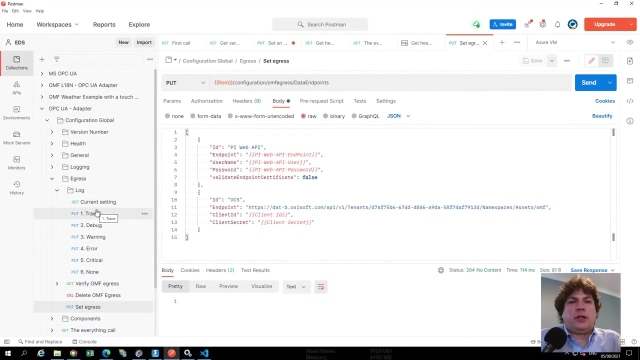 egress. there's one that's called global first systems, and then we'll see there's going to be one for other components, so, for example, the components related to getting data from this ops, upca, opc, ua server. but i have the ability to play around with how much i want to log that data. 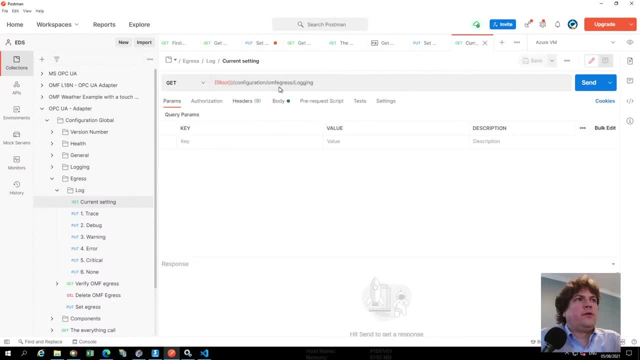 so here i can look at the logs and i'm going to. there's logs for several different of these and these different components of the of the editors in particular. here's how i would configure the. the logging for the omf egress endpoint is just omf egress login. 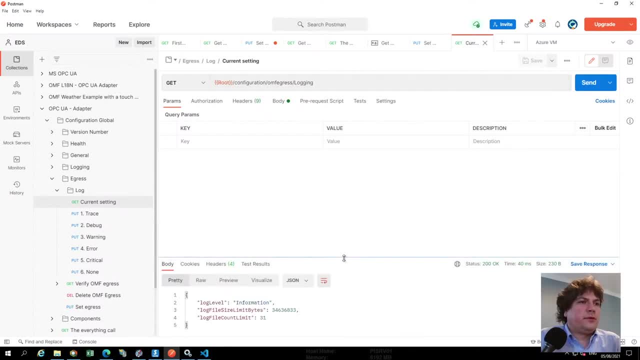 so these urls tends to be fairly obvious to do, very obvious to figure out, but of course we have the documentation about where they live and here i can see that i have the information. uh, the i'm logging at level, the information level. if i want to change these levels, if i 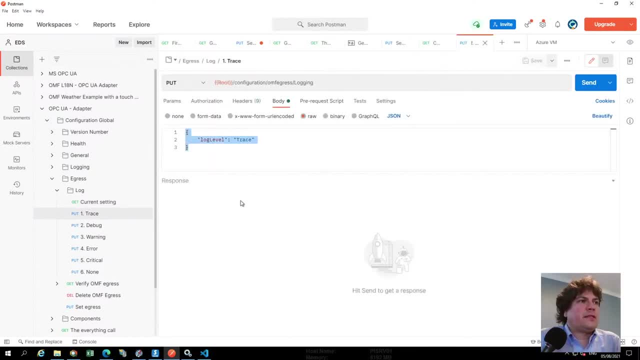 want to increase them, i can just simply send another message which will say: well, increase it up to the trace level, or increase that to the debug or warning level. i'm just putting numbers one, two, three, four, five, six here, just to remind myself that these are kind of. there's an increasing. 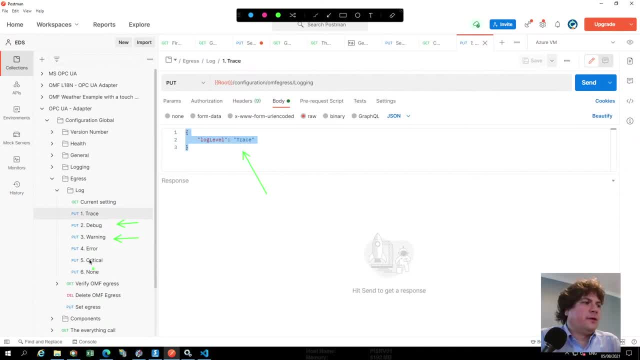 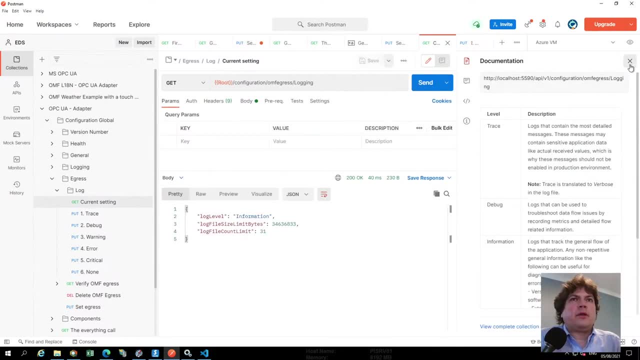 list, you know, traces the one that has the most details, six, which none has no details at all. so again. so here kind of a note that i've kept for myself is i can the um put the documentation inside of postman itself. that just reminds me of what it is here, but i can always, uh, go back. 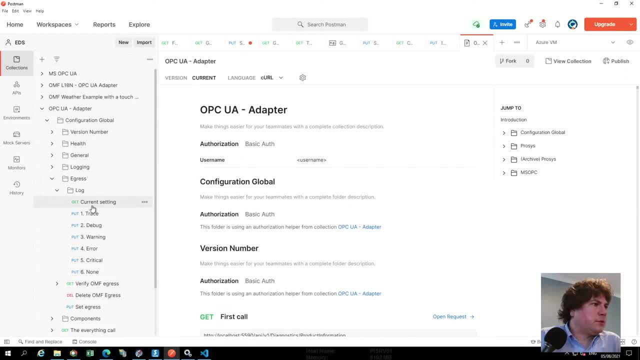 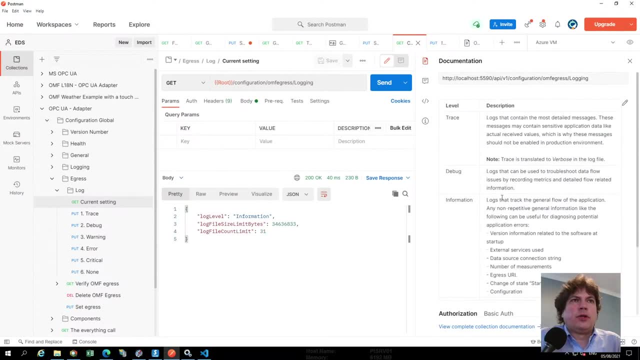 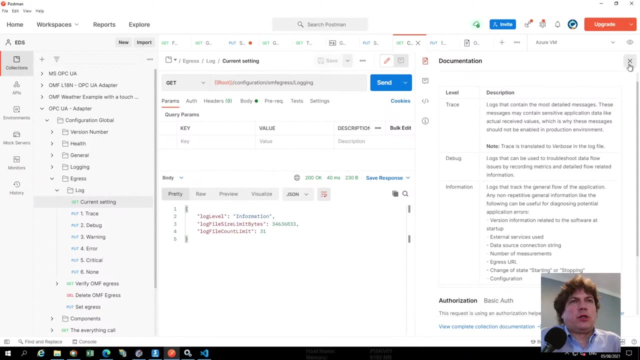 to the, the docs themselves, to look at it. oops, let me go back here. so yeah, so this is the, the documentation that i'm currently using, that i'm building up for myself for how i should configure the adapters so it all can live within this one tool here. 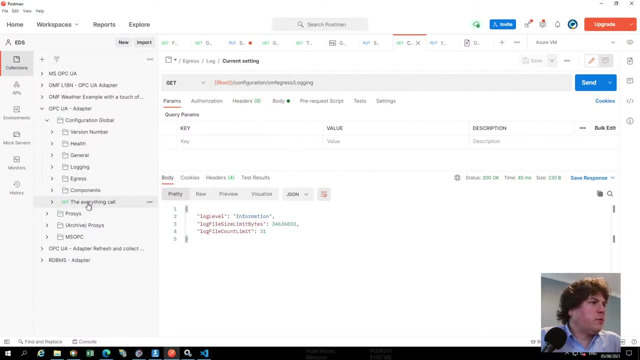 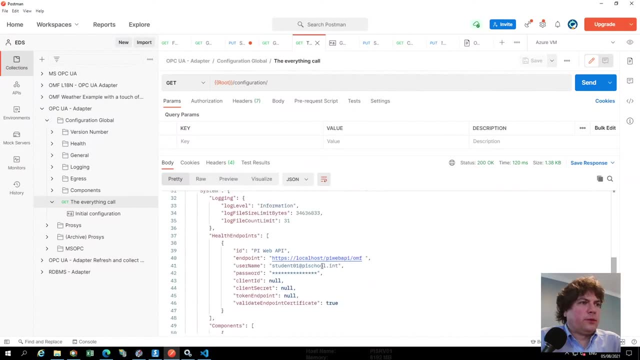 okay, and now i can always just verify again my my single call. so the call that contains everything and i can look now that i have my health point was configured and my perfect scroll up a little bit. my data endpoints are now configured where i'm sending data to pi, wave, api and i'm sending 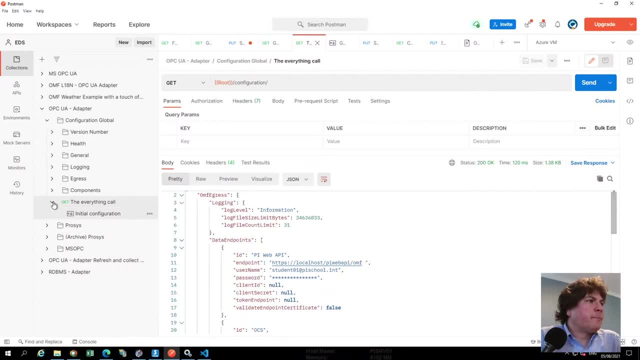 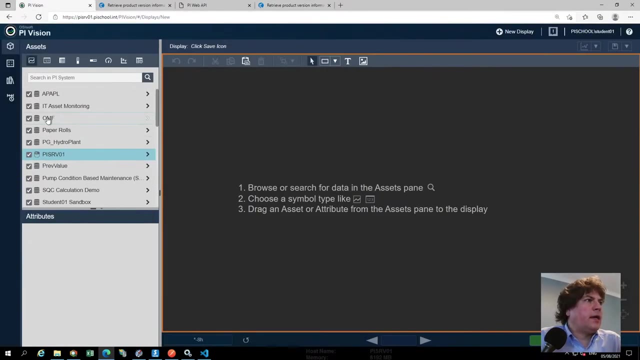 data to lcs. so now that i'm actually sending- i've configured this health data, maybe i actually want to go back to my pi server and i can see what the data is that i'm sending to the pi server. so to do that, i'll just go to my pi vision display and i'll go to a database that's configured. 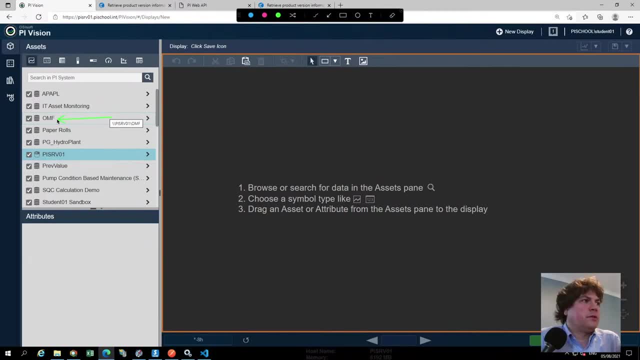 for receiving all types of omf messages and just to make it very clear, just called it omf, so i'll go to scroll down to omf. i see that there are objects created, there's assets created within my omf database and these are assets that are created. 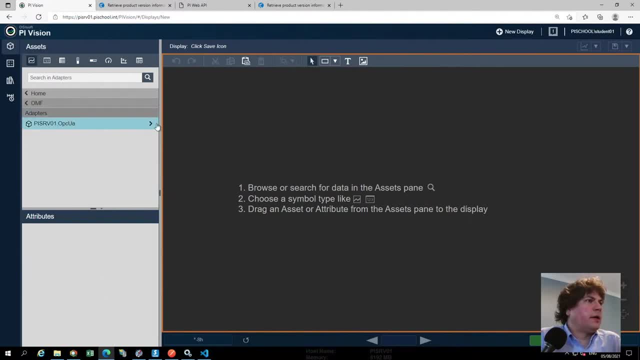 by the adapters. so i'll drill down to my, to the adapters, and i can see i have this opcua adapter which is the one that contains the information of one of what it's going to send adapters here. okay, so here is the, the level, the, the health information that the adapters 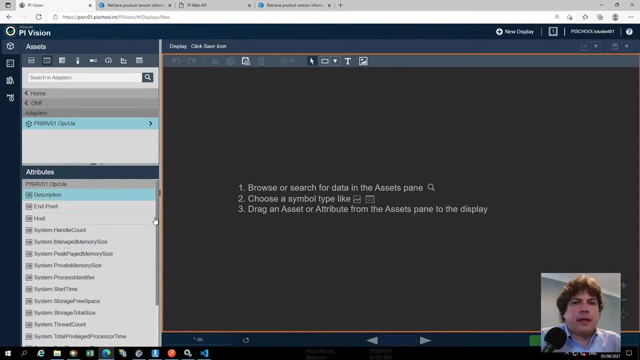 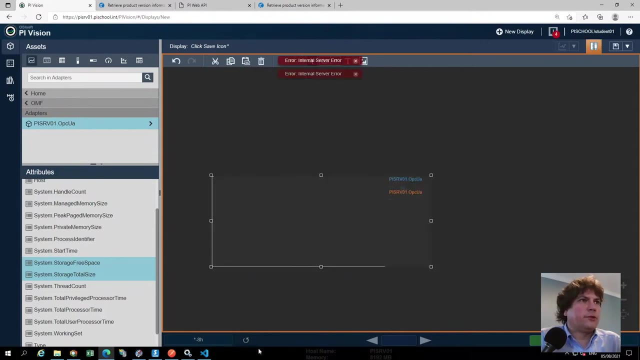 are sending um. let's just drag some in there in my pi vision dashboard to see what it's there you can see. for example, maybe since i know i'm going to be i'm configuring a data source, the information about how much hard disk is available should be important, interesting for me and okay. 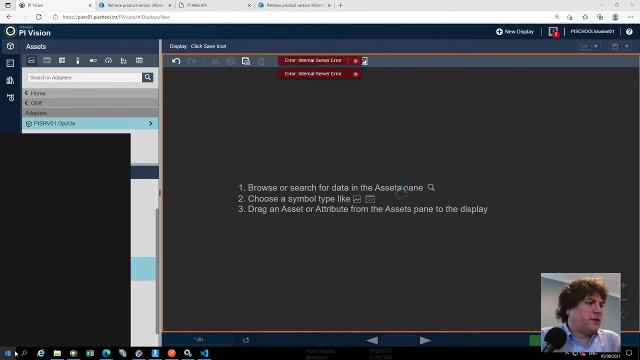 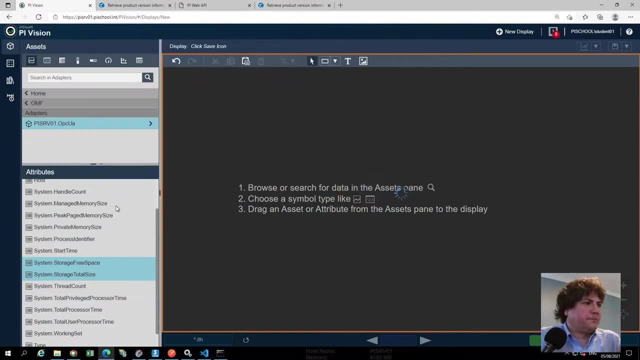 my opc. uh sorry, pi vision is not acting up, is acting up again, so let me just look at this again. i'll just reset it and look at it in a minute, but here these are the content, the common health, the data that i would like to see as we're waiting for my pi vision server to go back. 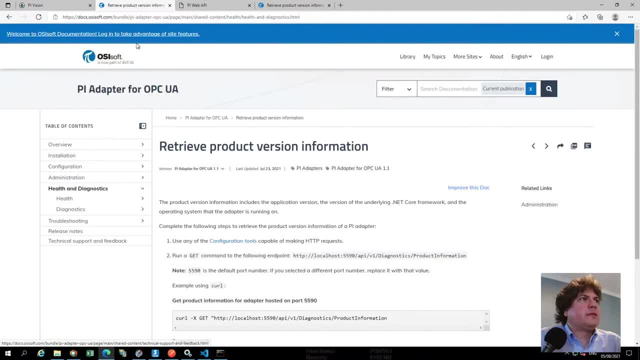 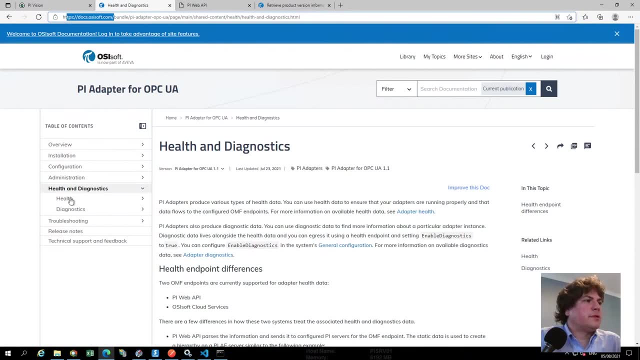 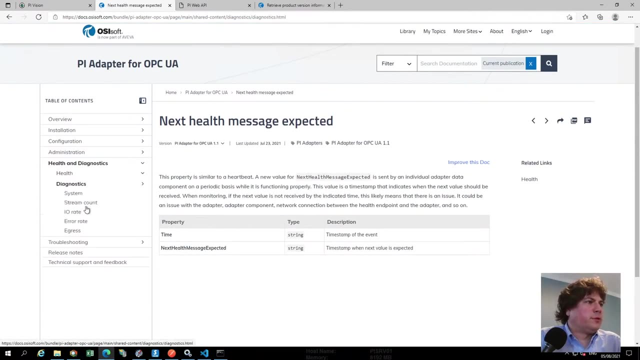 up. i'll just look at the inside of our website. so docsosisoftcom has all the documentation related to couldn't adapters here. i can look at them and look at the health messages that are going to be sent. so, for example, what are the? you know what's the af structure that's going to be built? 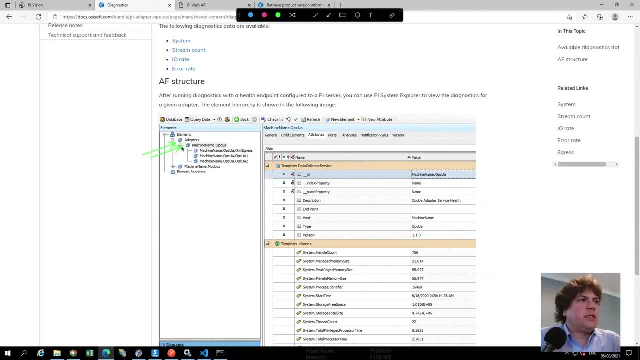 so i have the adapter on this machine. these are going to be all of the different adapters are installed on this machine. i have, you know, the adapter and here i can see all of the kind of the, the data points that are being sent. so all of the, the data that's being sent to this, this adapter. 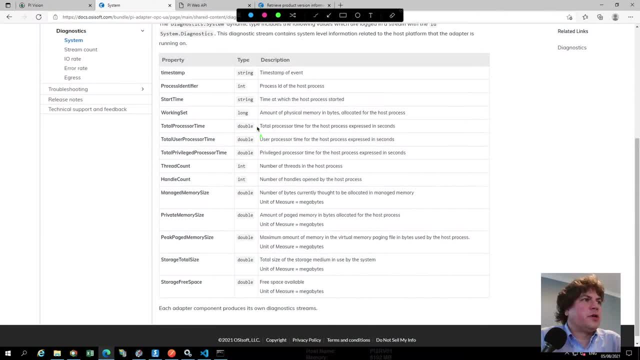 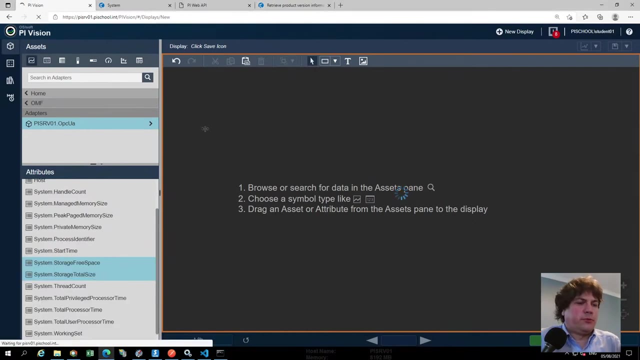 and in particular i can look at the, the exact definitions of of memory that's being sent uh hard disk that's being sent here and hopefully my pi vision server is back up. so once it is back up i'll be able to at least show some trends about how much this space is remaining on my uh, on this vm, and how much this. 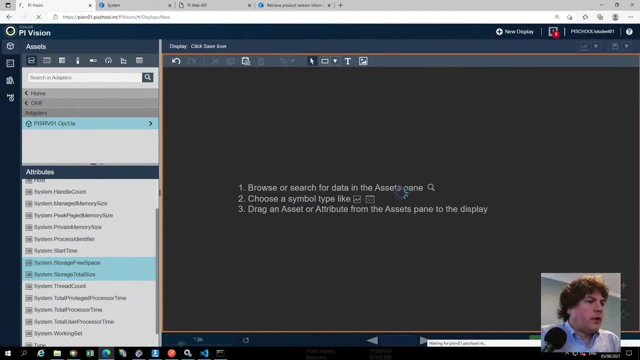 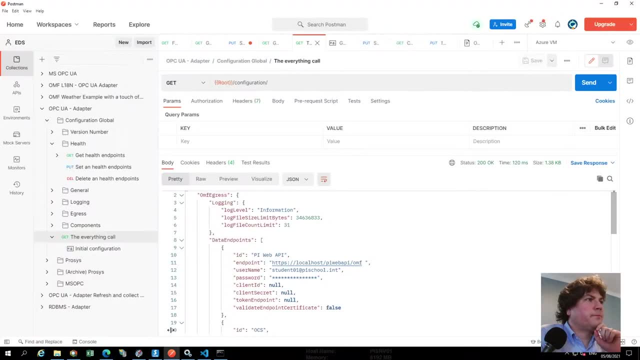 space is being used by the adapters. if my vision doesn't collaborate, i'll just continue on. okay, so, okay. so here is now. i'll go and start configuring the component. um, so, for the pc array adapter, which means, what do i need? is that i first? i have to be able to say to the adapter: from now, 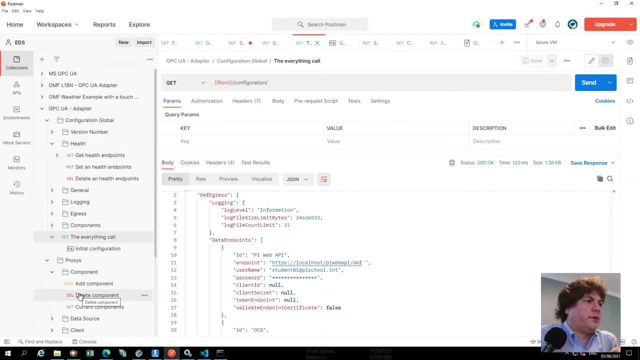 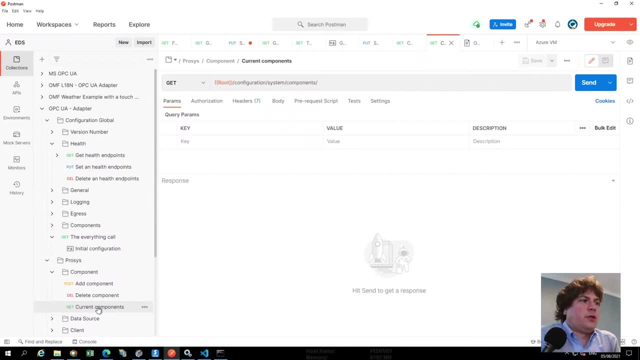 on, you'll be collecting data from a new, new source of data, and these are going to be called components. so from now on, you will be getting data from a pcua server source. okay, so through here. what i'm going to do is add a new component. so the url is very simple. it is called simple uh system. 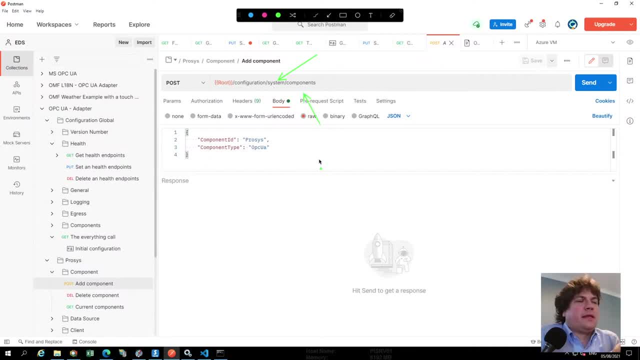 it's called components. so i'm just going to slash components and i'm going to be sending a certain data which is the component is opcua. so this is going to be specific to each of the adapters: what the name is going to be and the component id is going to be the kind of the metadata of how i'm 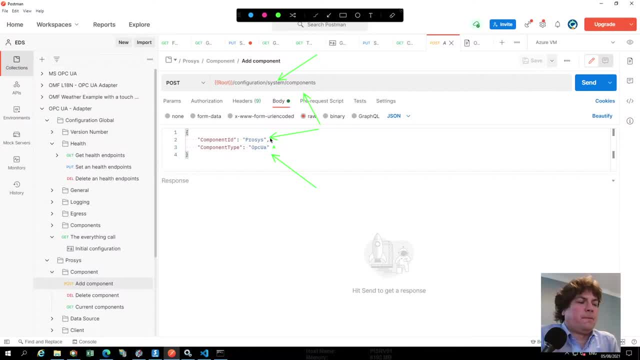 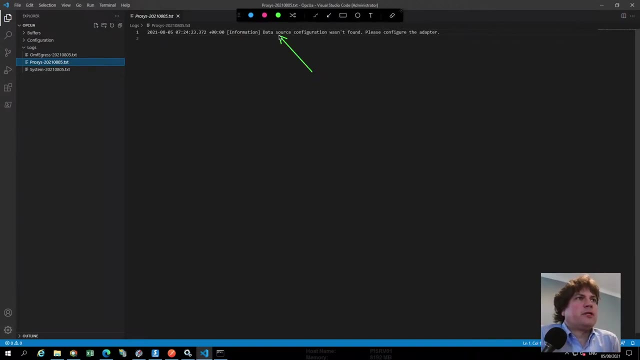 configuring this adapter. in this case it's just going to name that i'm giving this component, so in this case it's process. so i'll create the process component and i should be able to now see there's a new log being attached to that and it's giving me information that 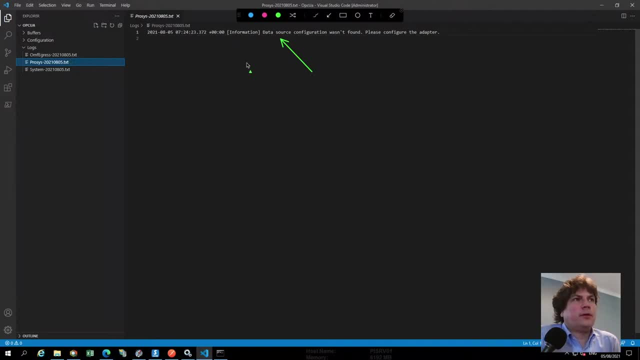 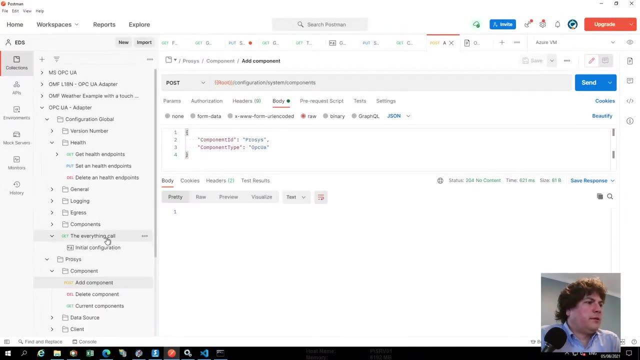 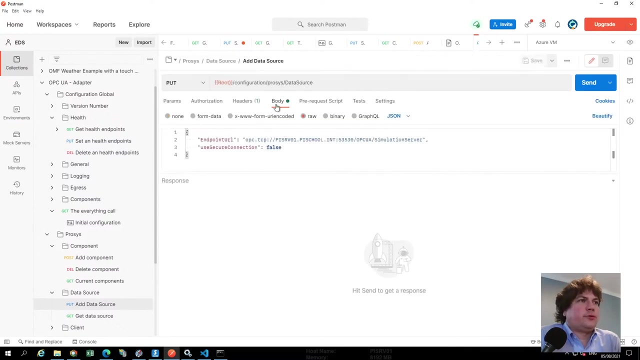 while this, this adapter- sorry, this component- is configured, it doesn't have a data source, it doesn't know where it's going to be pulling the data from, so i'm going to tell it this information, so i'm going to add to the data source. add the data source information here. 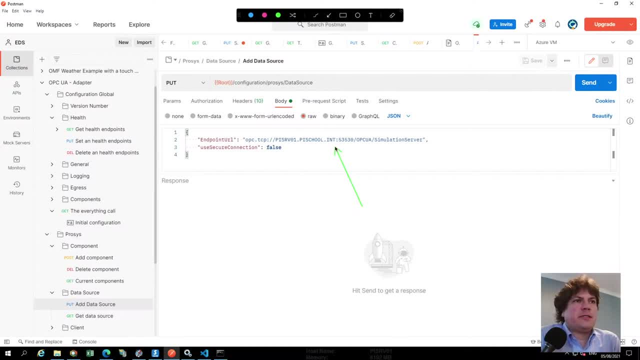 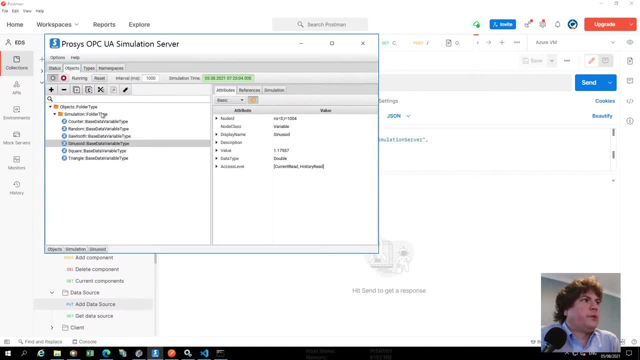 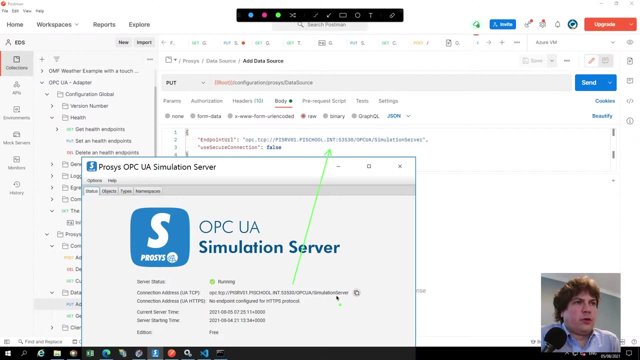 so i just need very simple, a little bit of information, which is where is the opc array server located. and this information i could get it very easily from my opc array server, because it's simply, you know, the string that the opc array server defines. this is where simulation server is. that's the url that i use. 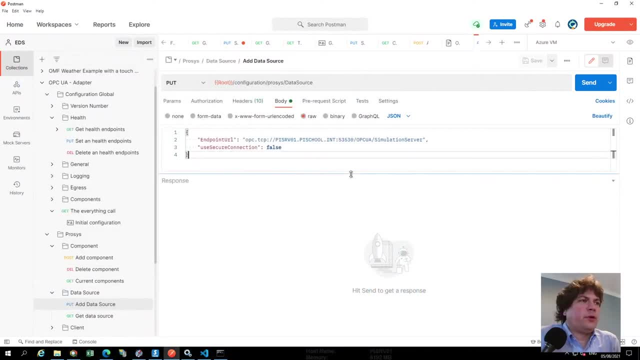 and since i'm not using any type of security, what i configure each thing. so i'm just telling it again: don't use security, so i'll hit send and again it's not returning anything. the adapter just received a request, it's now happy and it's working in the background. if i want to look at what it's, 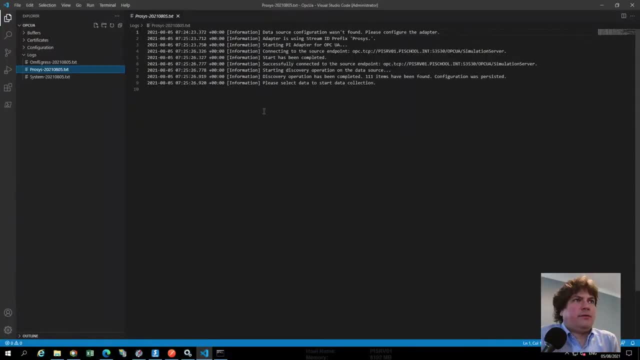 working on. i can then start looking at the the logs level here and the important things about the logs here is so if i want to look at the log level, i can just hit send, send and automatically it different ages come, and then it automatically comes back to training. 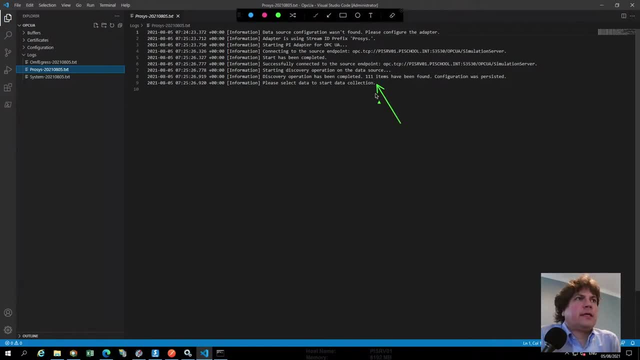 the adapter just to get All right. so i've got these methods being running. so right now for that long list. so if i want to, the important things about the logs here is that this information that it did discovery on the server- so doing discovery means i was the adapter- was able to connect to the opc ua server. it now 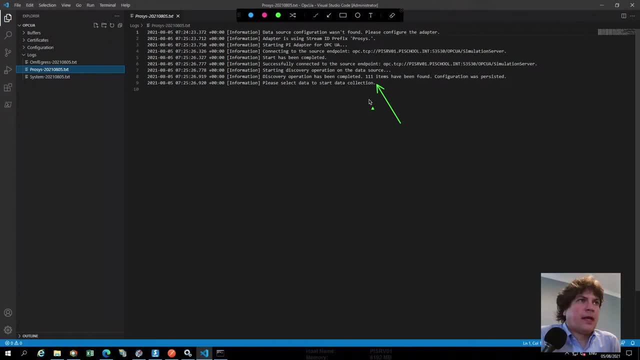 started to browse the information that's in the opc ua server and it found that there's 111 tags that it can do, and it's actually now telling me the next step for what i should be doing is i have to select the data to actually start the configuration. okay, so let me look at the 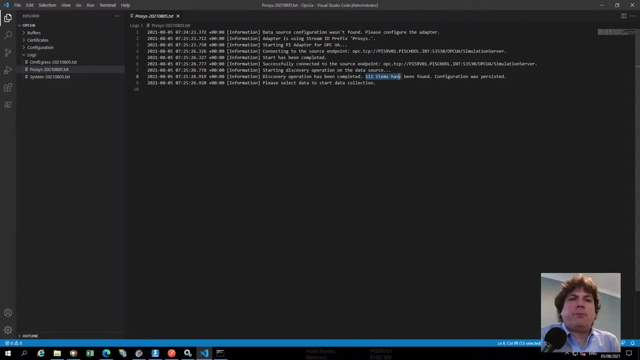 and it actually, since it was able to browse the information, it prepared a file for me about what data, what data is available and what data you want to collect. so here i can go to the configuration and i'll see this. there's a file here that's called data selection. 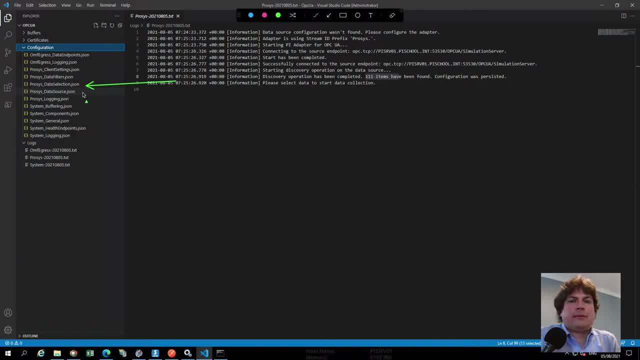 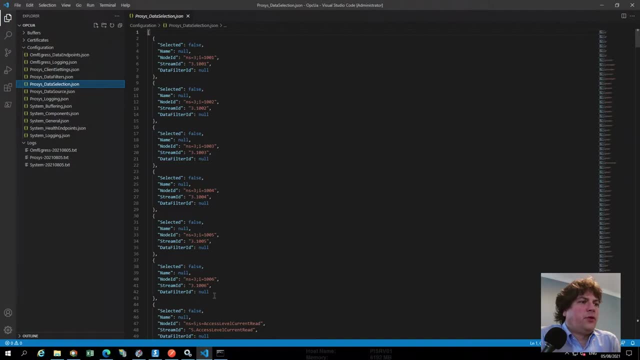 which contains all of the information that the opc ua adapter was able to find on this opc server. so if i click on it here, i can see that there's a json object of of tags or part of the opc ua server that i can use to do data collection, and what i'll do is. 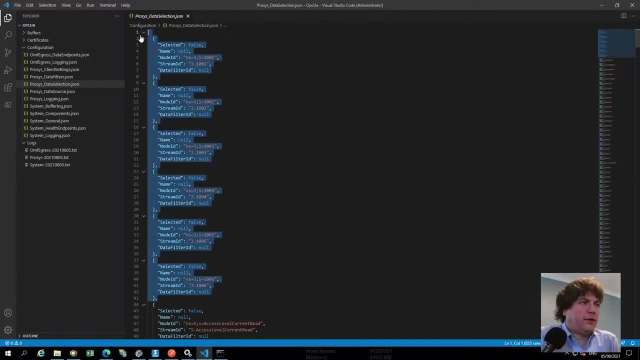 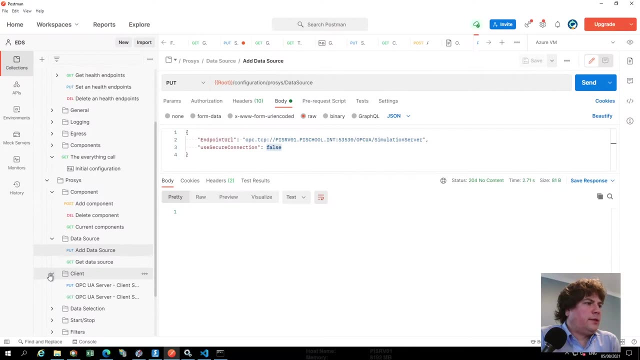 actually just select these first few ones here. i won't select the entire file and bring them over to postman and put that in my data data selection request. so i'm going to go here to select data. i'm going to tell it from now on: this is the data that you want to collect. 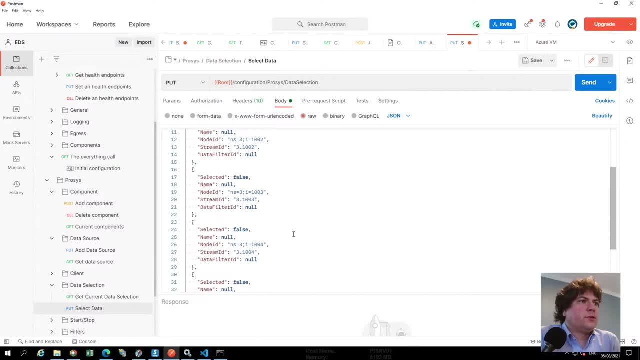 okay, so there's a few details here let's first look at. one important notice is these have to be all json objects. postman is then telling me here that i have. you know, there's kind of syntax error in my, my json object, that it shouldn't end with a comma, so i'll just close that, put a square bracket. 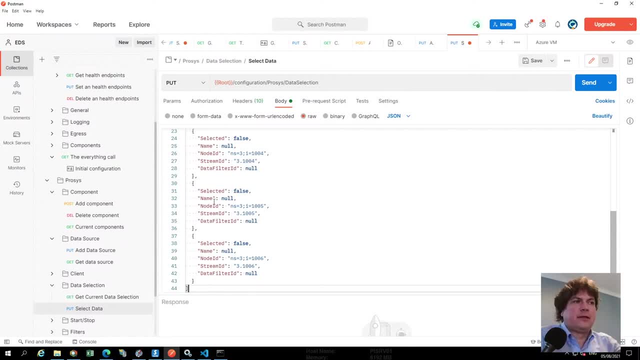 there due to say that actually this is the entire list of the json objects that are there. let's just look at one of these objects. oops, no, i didn't turn this off here, so the first part that's very important notice is the this thing called node ID, which is on the OPC UA server. where am I going to retrieve this? 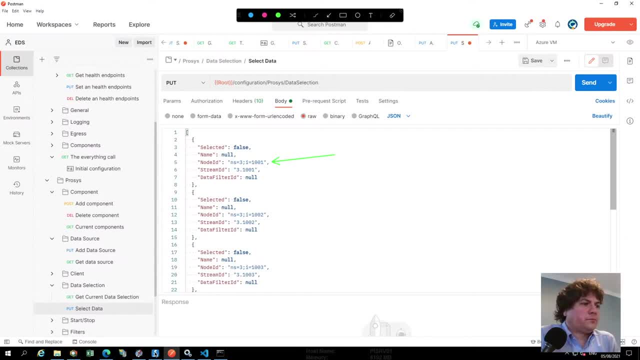 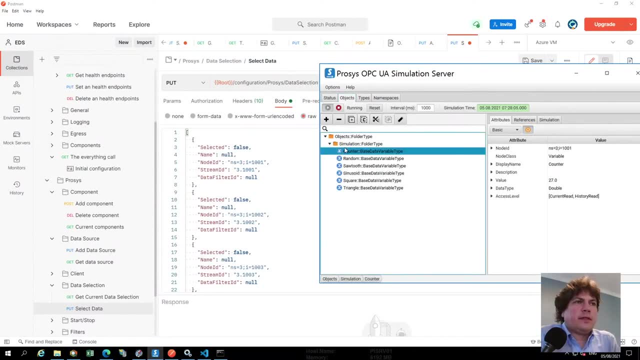 data. and if I look again at the OPC UA server here I'll see. if I look at the names, yep. so I see that this counter I can see that it's node ID is namespace equal to three, index is equal to 1001 and that is this information here. so the 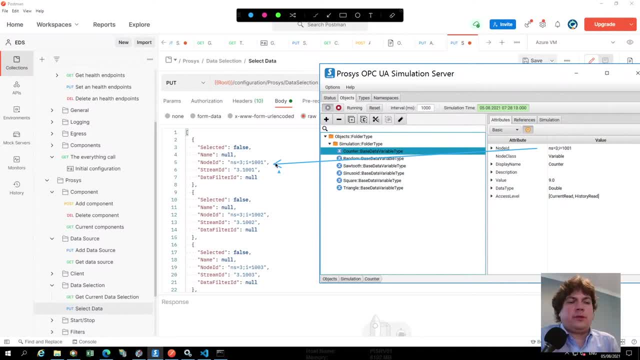 OPC adapter. when it browse the OPC UA, the OPC UA server, it picked up this information and allowed it to be here. the next one is the information about a stream ID, and a stream ID is information about: well, what's the name that I'm going to be sending it when I send to the data, to the data archive? what's the? 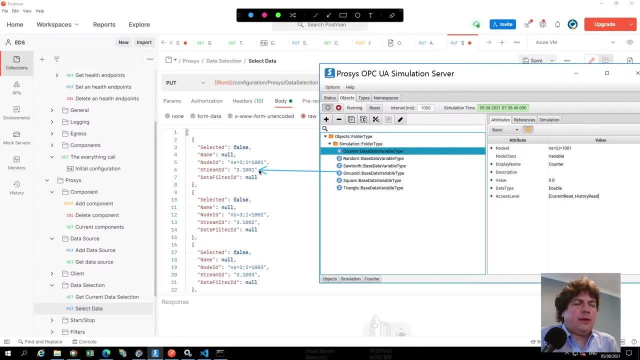 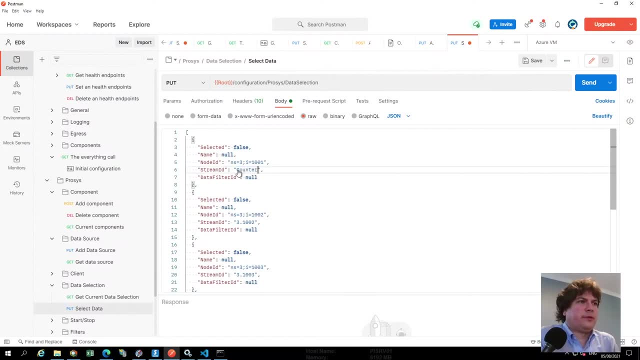 name that it's going to use for that. and of course the name in the data archive means the tag name. so here I can just rewrite it, that this is going to be, you know, for example, counter, and that's going to be the name of the, the stream ID of the of these counter. so here, 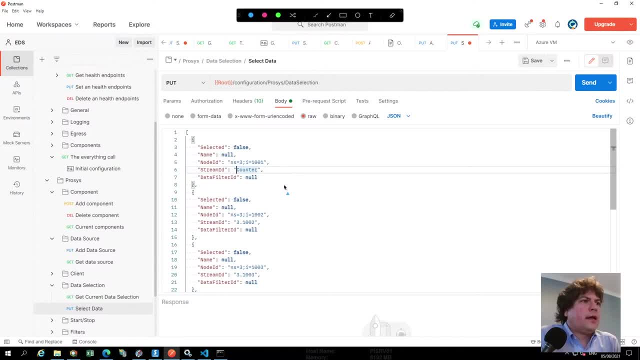 actually I'm gonna. yeah, just counter is gonna be okay and other information here is selected is so, even though this piece of data is in this file, is that data that I want to collect from OPC UA server and send it to PI or send it to OCS by default? it's false, because here you. 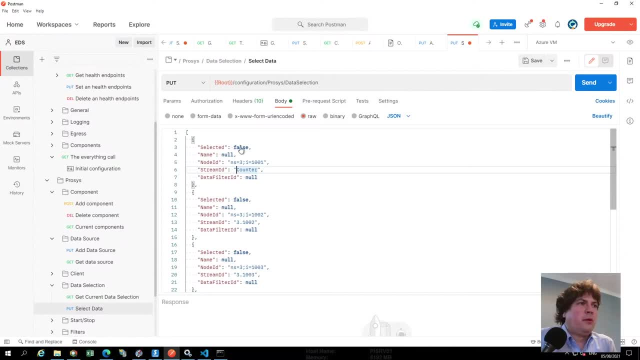 might want to contain a list that contains everything, the OPC UA server, but only selectively send the data. so this one, I'll just send it to true. the other information is a data filter and I'll show that in just a minute. it but it's the ability to filter in from to apply kind of an exception, filtering for. 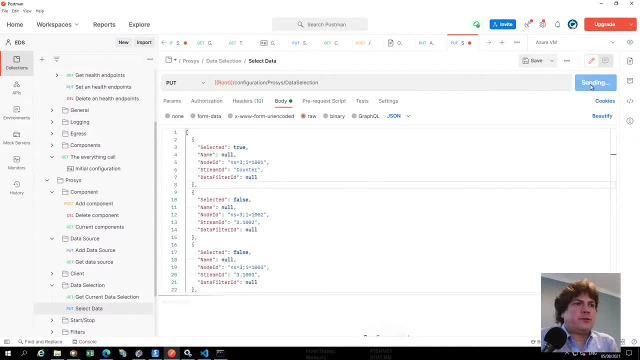 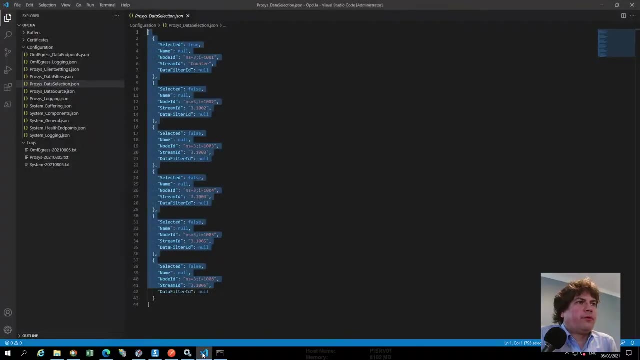 adapters. it's very similar to how we do receptions for interfaces, but it has its own variation on that, that first shade team here. so here I can see again no problem with the request and I have sent it. but if I want to look at the work that's being done behind it, I can. 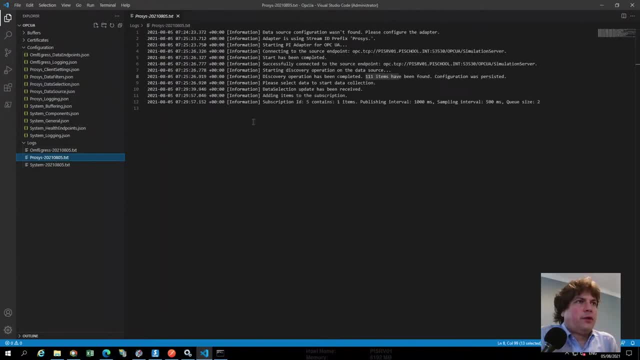 go over to the logs here. the log says: I can see that when I hit send in, postman it the adapter is known as: oh, there's a data selection. I'm gonna look at what it's going on. okay, and what I was gonna do is I'm gonna subscribe to one item in my OPC UA server. so from now I'm 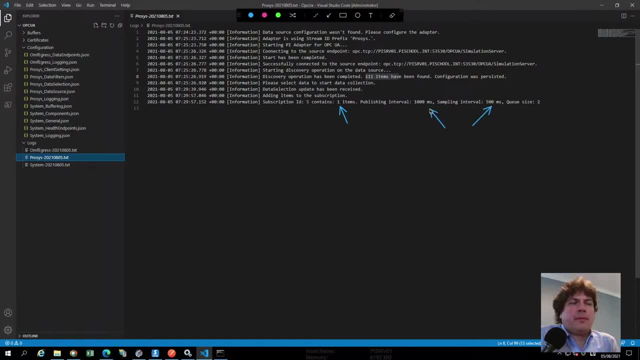 collecting one piece of data and there is more information about how quickly I'm gonna collect the data from the OPC UA server and how quickly I'm gonna send that to the PI server. so sampling interval means I'm looking at the OPC UA server twice a second to collect data from it and sending that data um. 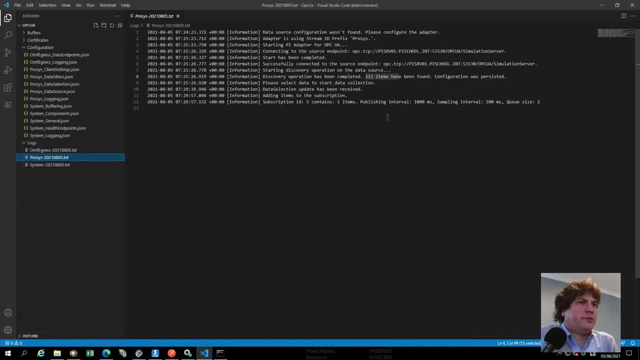 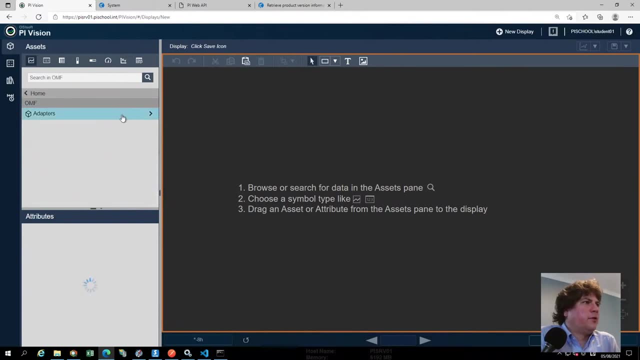 bundling up two events together and battle harbor, Everything, Ac� that to the Pi server here. Okay, let me go back to Pi Vision and let's actually look at this data First. let's look at the health data and let's see if that is in a better state. 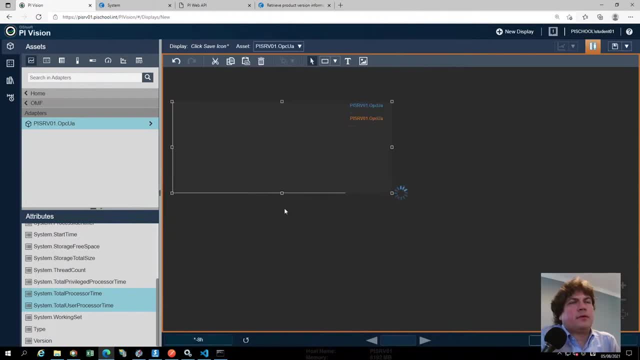 And hopefully, if I can drag data here, it will see trends. I'm crossing my fingers. there we go. Okay. so obviously I've done that before. So there's data in the past, but let's look at that for the past 30 minutes. 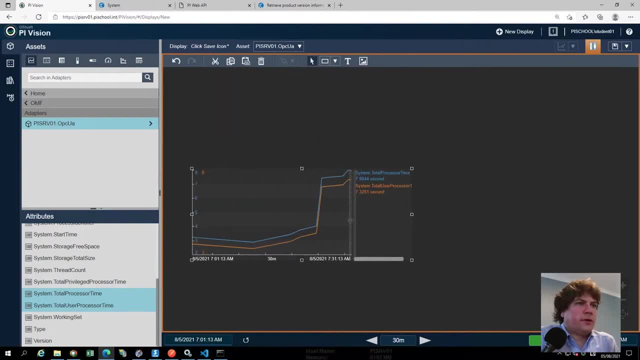 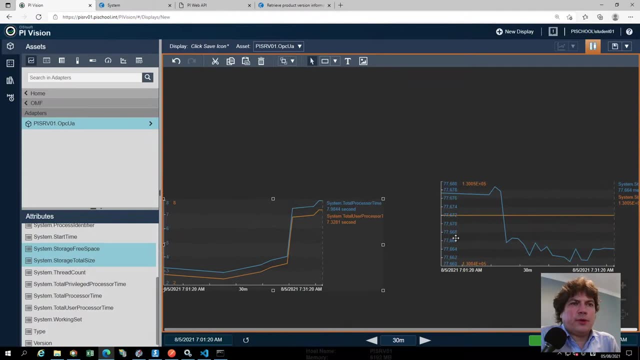 All right, so here is the total amount of processor time used. Let's see maybe sorry. yes, free storage, That's maybe more important, since I'm doing it. adapter. I can see my storage is slightly going down, but I still have lots of rooms. 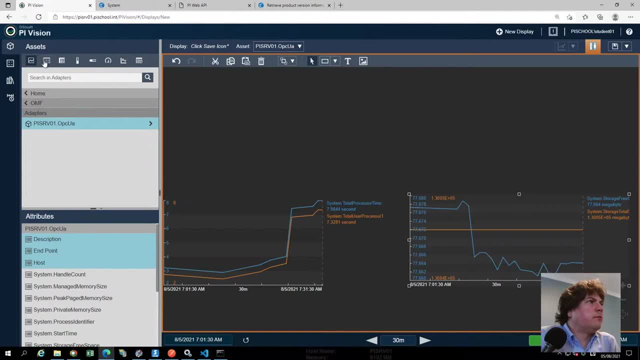 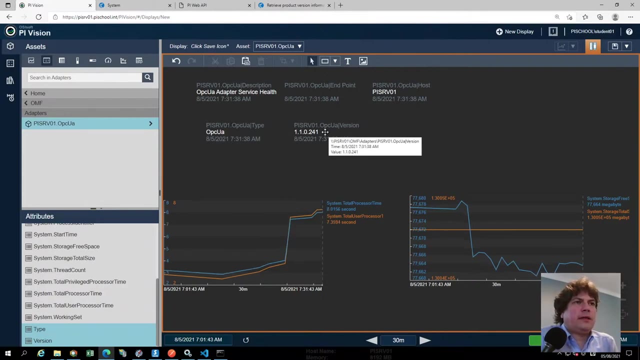 I can see information, metadata information. I'll just put them here: adapter, health and so, for example, type in information, So again. so these are metadata information about the OPC UA adapter that's stored inside of my AF hierarchy, That, and I'm sending data here. 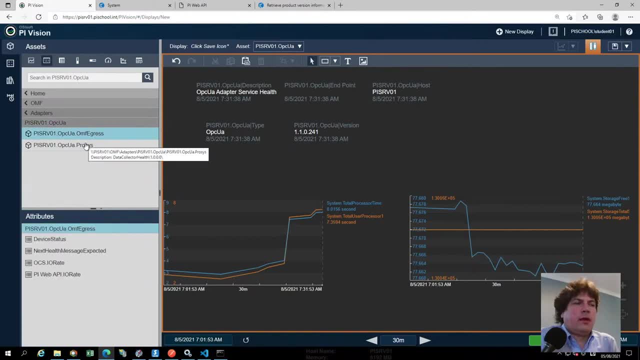 I should see it more details about these end points that I have. so this is the two components. So the component that sends data out, it's reporting itself and the data that's connected to my Provisys server is also getting data. Yeah, 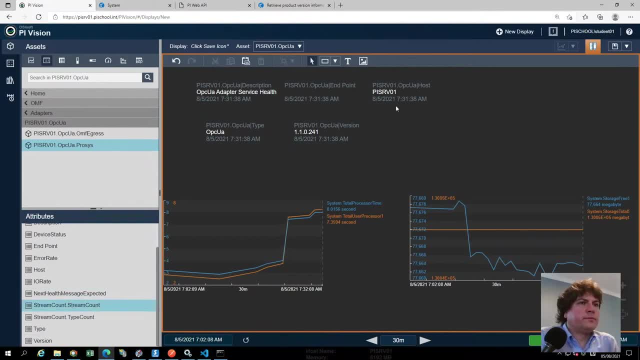 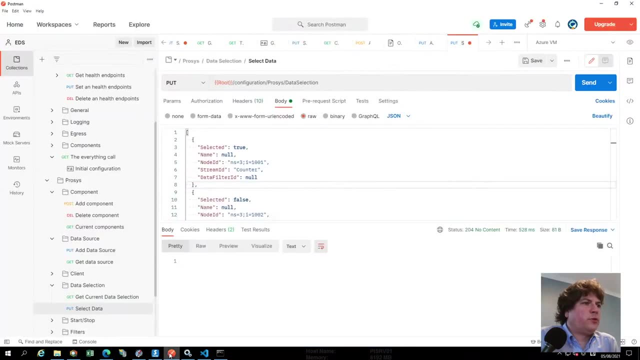 So I should see stream count. So I'm only getting one value here and it's reporting one value here. Let's just tweak it a little bit. I'll be collecting data for this other point here, Say when I get this one, and then look again. 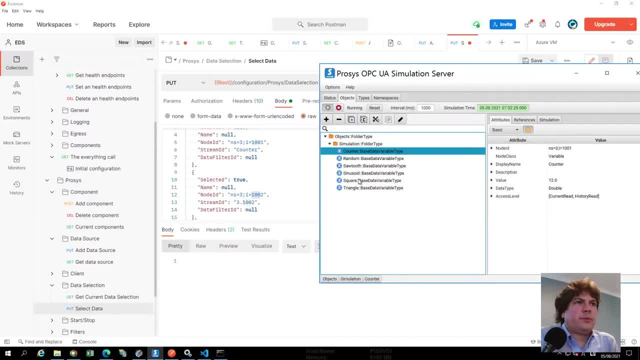 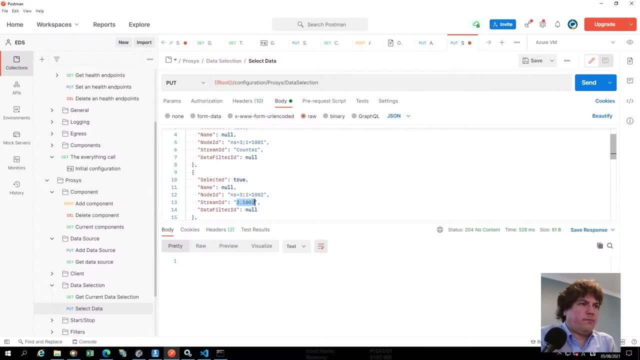 what was one one zero two? I can look at the OPC UA adapter configuration and see that one one zero two was random. So I'll just create something that's called my random tag. I'll just use my cause. I'm pretty sure I have something called random. 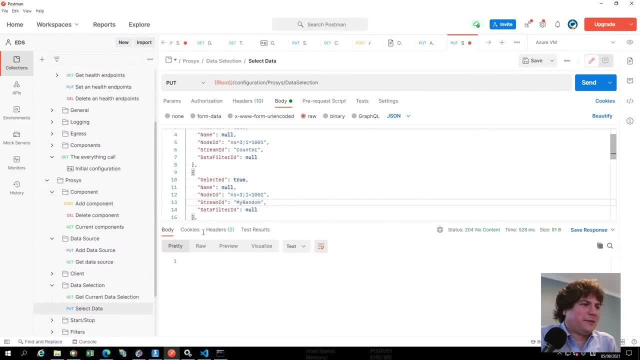 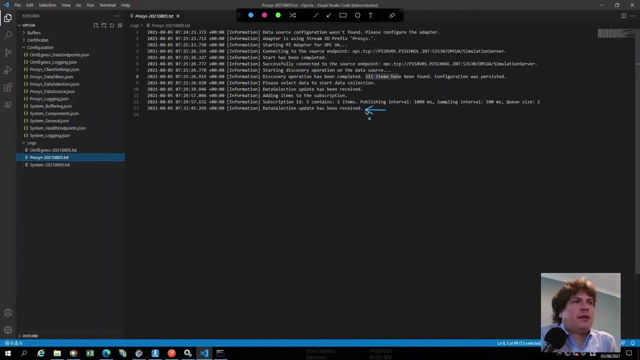 on my system, So I'll just try to prefix it and hope I get something unique here And here again. if I look at the logs, I'll see that there is a new met data. selection of data was received in a few seconds. 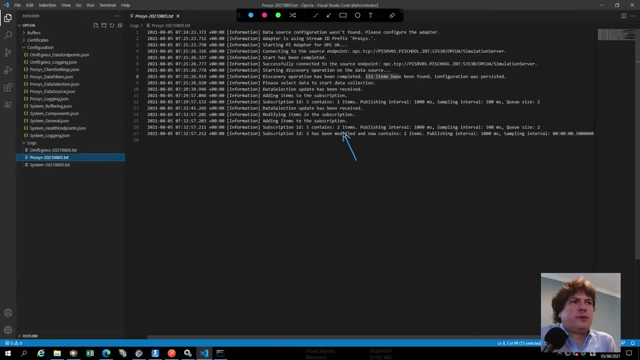 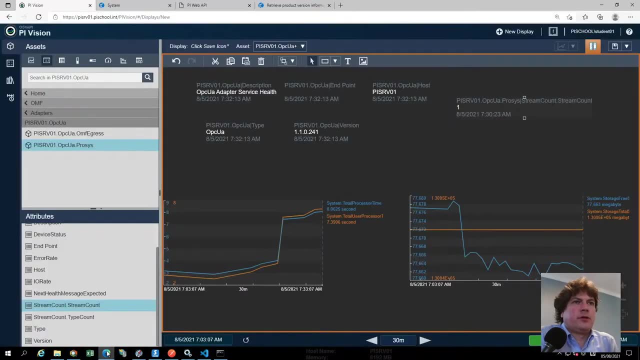 The adapter is now starting to collect data from this OPC UA server. So you see, as I'm now collecting two items from this OPC UA server and this is gonna be reflected in the KPI, This will be updated in just a minute to show that I'm collecting two streams. 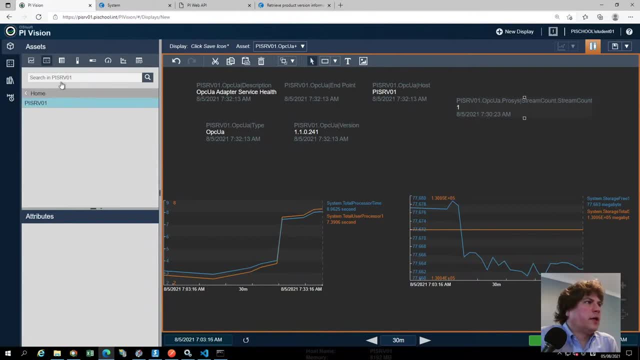 But in the minute, in the meantime, I'm gonna go to my PI server and look for my tags. Hopefully my random tag has been created by now. Yep, I can see the tag. The naming is: it contains the component and it contains this name of this random. 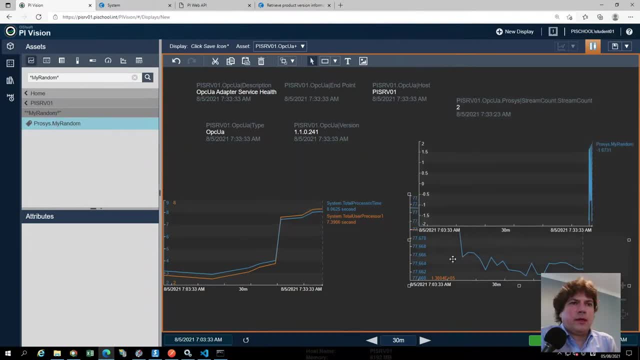 I'll just drag this up to somewhere else on my screen And I can see that I am now sending this random data here. I think I had something called counter as well. I'll just look for counter, drag this up here and I can see that the counter one is getting data as well. 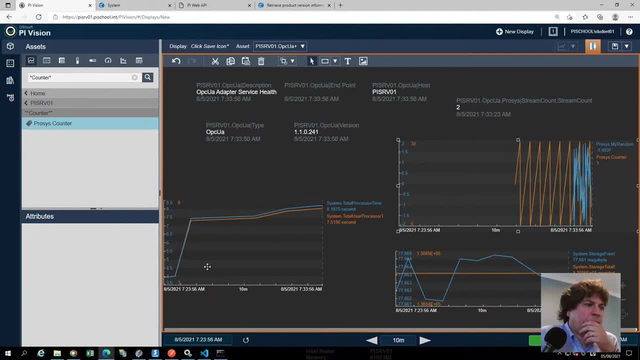 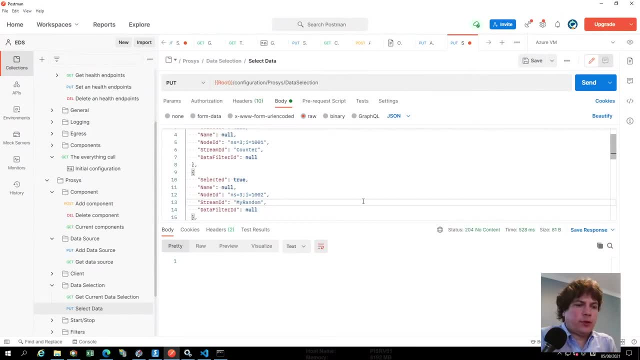 Yep, okay, so my counter just goes up and down. Okay, so that's very convenient to do And okay, so that's fairly straightforward. I can see that I think to do it And I'll be going over just over the concept of filters. 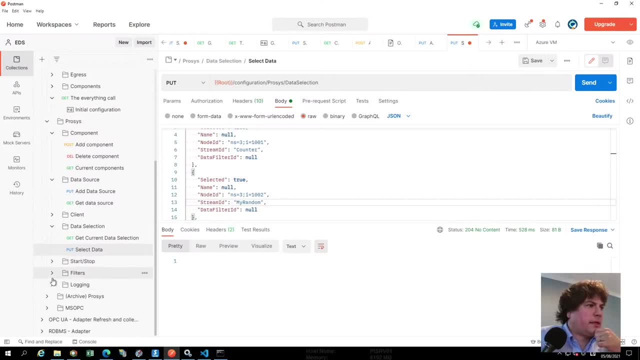 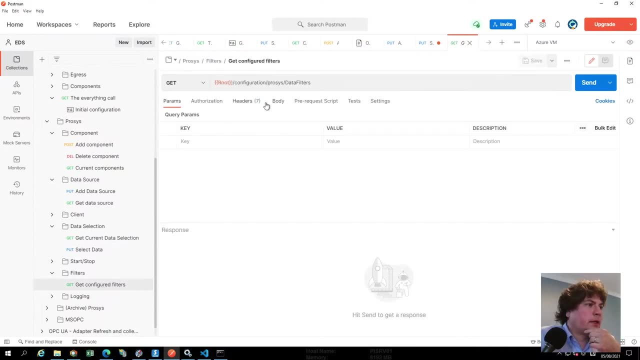 and then end this stream. So if you have any questions, you can just ask them now And I'll get to them just as soon as I describe what the filter functionality is. So here I can look at filters. Filters are this ability to remove the data. 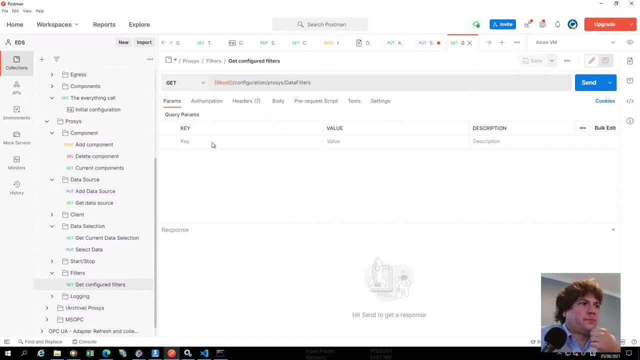 that shouldn't be sent to a PI server if it has no value. And we do start with one basic filter applied Here. there's already one that's configured And I can look at the definition here It contains: its name is duplicate data. 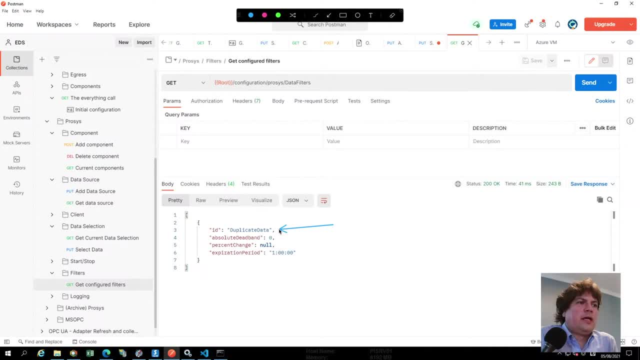 which simply means: okay, you know, any data that's identical to the next data shouldn't send it. And the configuration is pretty simple. I'm just asking it to absolute dead band of zero, which means if the data has not changed. 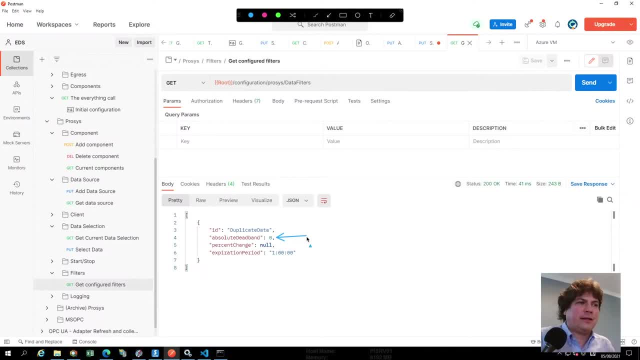 if it's exactly the same value as the previous one. not that there's any delta, it's exactly the same send. do not send the value, But I have an expiration period. It means if there's the same value and I get the same value continuously for an hour. 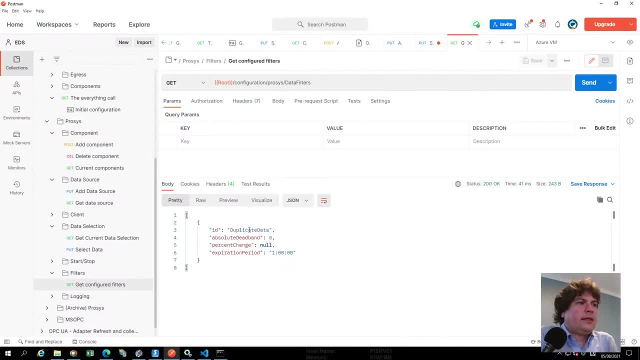 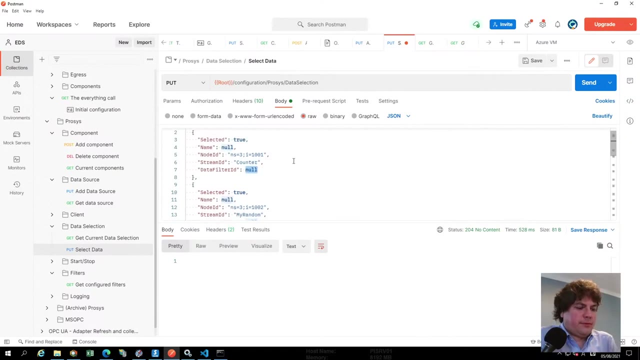 I should do send a value there- And this is the policy that I'm using here- for kind of a default value. And now I can go back to my data selection And actually when I specify a data filter here, I can actually specify your counter data. 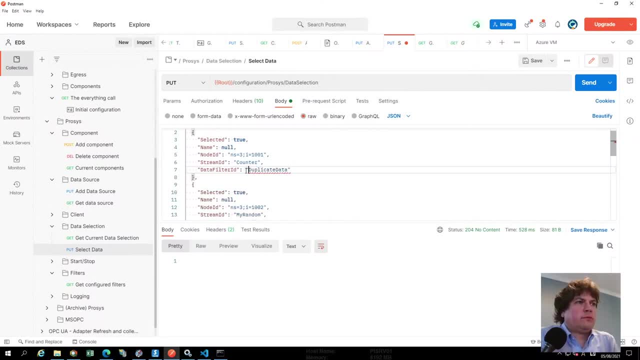 You're going up and down. Okay, it's actually sorry. the counter, since it is actually an increasing line, all of the data will be compressed. It won't be except so maybe I could do, maybe something's clever. 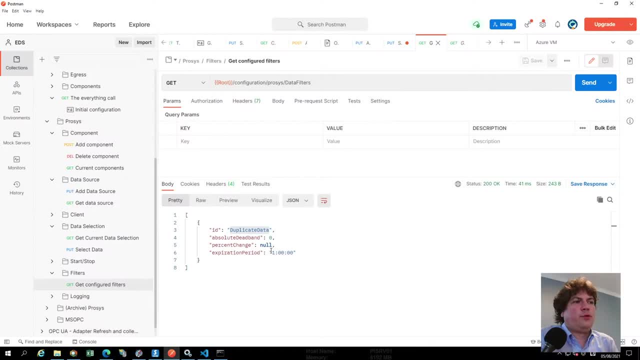 So I can say, for example, actually don't send every single value. If you're changing more than twice, then it actually sends the data here. So I'll just apply that here. I'll just create a new, a new one. 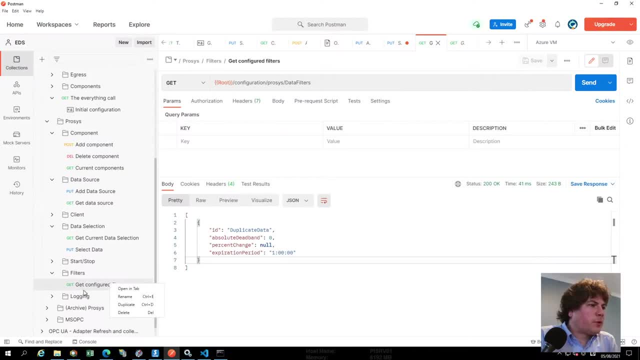 Okay, Yep, So here I am to create a new request. here I'm only retrieving the data filters. I'll just create a new request that sends data filters. So I'm gonna be sending information about the data filters. I'll just say put. 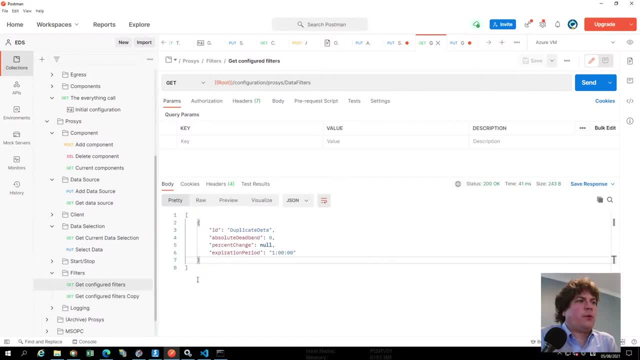 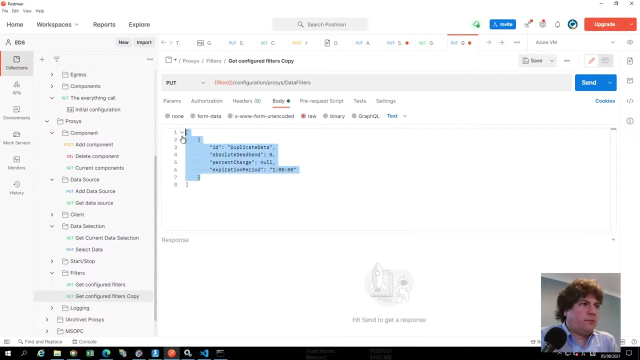 So put is gonna go over the entire request and remove everything else. So I'll just grab here and say that from now on, what I'll be sending is all filters, And the filters is gonna be duplicate data, Say, let's say, one engineering unit. 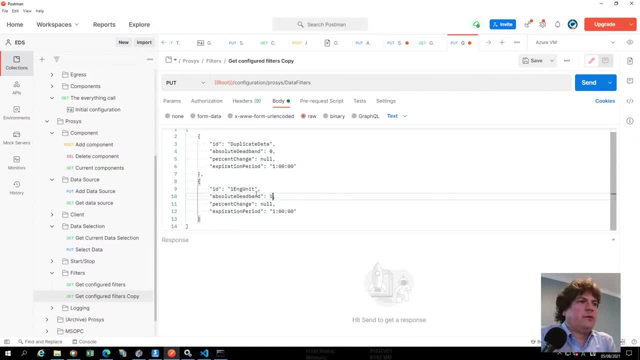 That's gonna be my name If it changes by one unit. if it only changes by one unit, do not send it. So that's gonna be my engineering data here. The data here that I'm configuring is about how do I want to send the data.